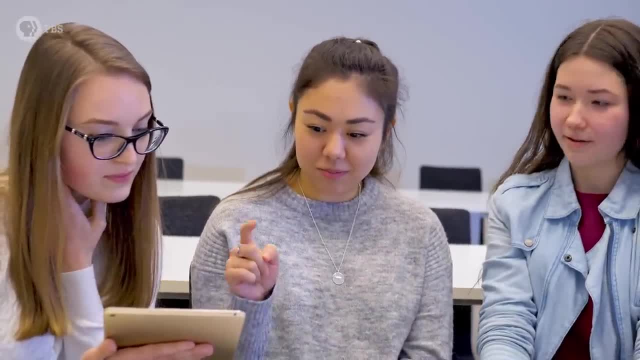 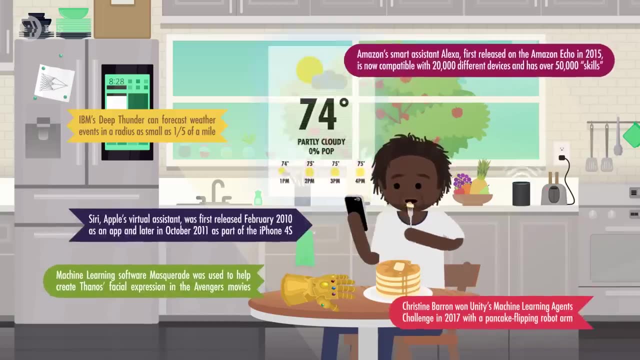 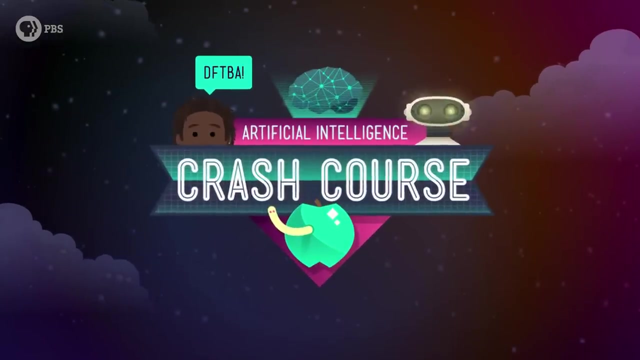 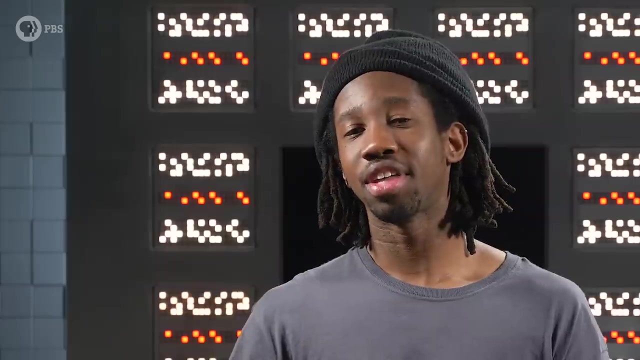 sometimes we even get a little help with our Spanish homework from Google Translate. So today we're going to explore the field of natural language, Natural Language Processing, Natural Language Processing, or NLP for short, mainly explores two big ideas. First, there's natural language understanding, or how we get meaning out of combinations. 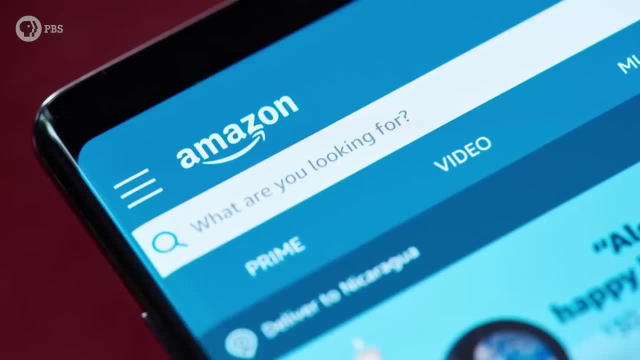 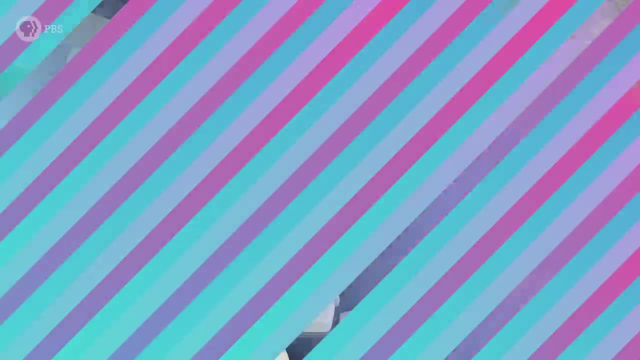 of letters. These are AI that filter your spam emails, figure out if that Amazon search for Apple was grocery or computer shopping, or construct your self-driving car, how to get to a friend's house. And second, there's natural language generation, or how to generate language from knowledge. 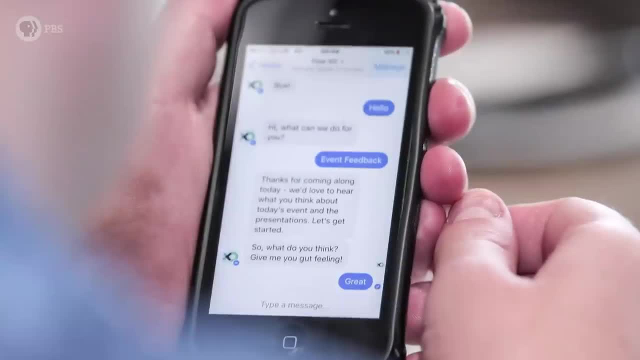 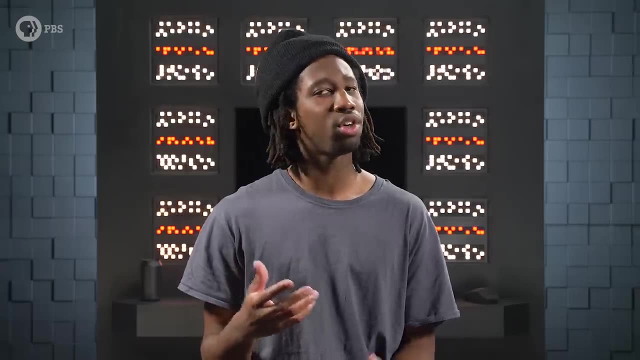 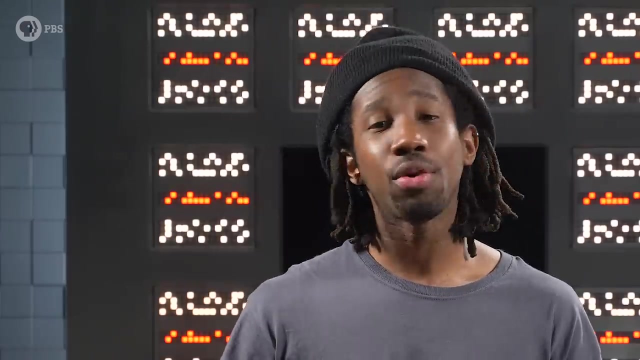 These are AI that perform translations, summarize documents or chat with you. The key to both problems is understanding the meaning of a word, which is tricky because words have no meaning on their own. We assign meaning to symbols To make things even harder. in many cases, language can be ambiguous and the meaning 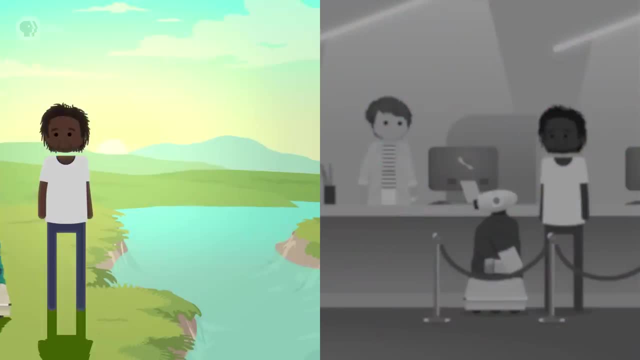 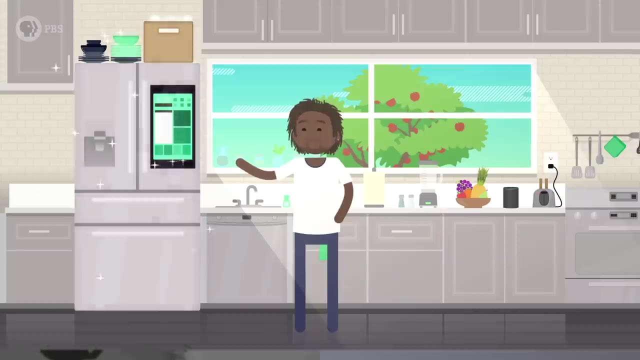 of a word depends on the language. It depends on the context it's used in. If I tell you to meet me at the bank, without context, I could mean the river bank or the place where I'm grabbing some cash. If I say this fridge is great, that's a totally different meaning from this fridge. 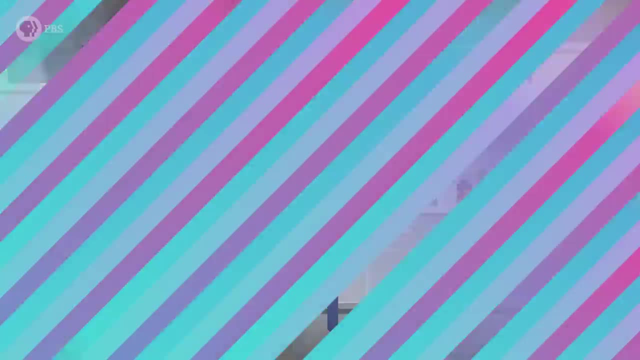 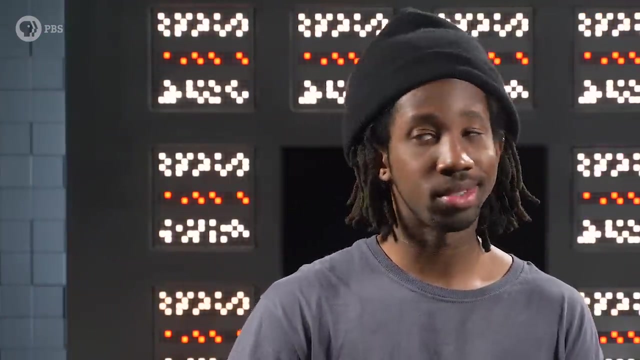 is great. It lasted a whole week before breaking. So how do we learn to attach meaning to sounds? How do we know great means something totally different from great? Well, even though there's nothing inherent in the word cat that tells us that it's. 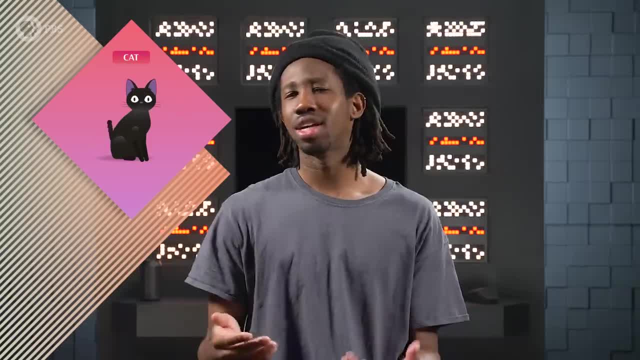 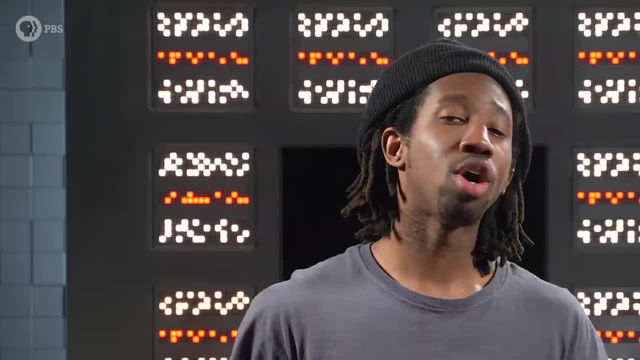 soft, purrs and chases mice. when we were kids, someone probably told us that this is a cat or a gato, maul, billy or ot. When we're solving a natural language processing problem, whether it's natural language understanding, 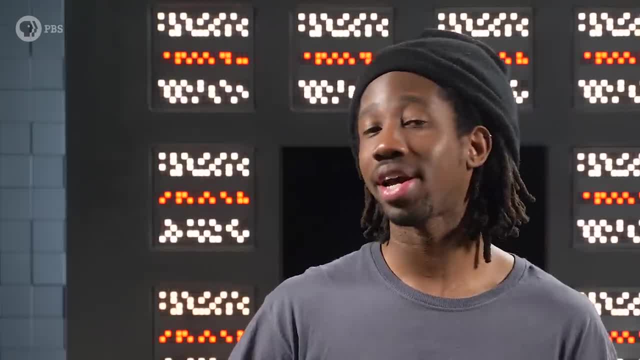 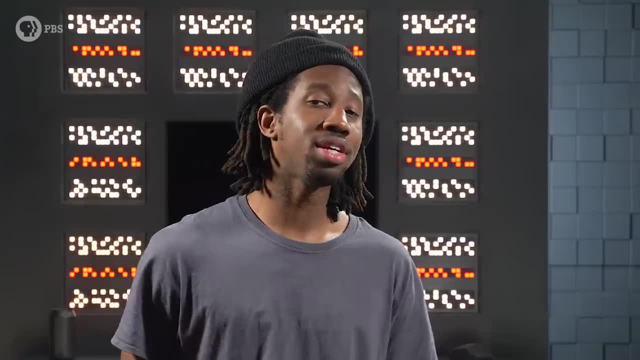 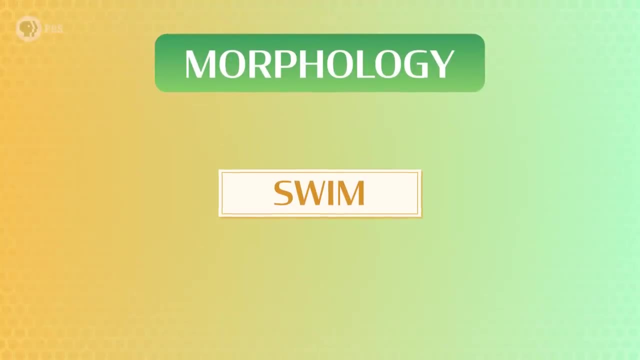 or natural language generation. we have to think about how our AI is going to learn the meaning of words and understand our potential mistakes. Sometimes we can compare words by looking at the letters they share. This works well if a word has morphology. Take the root word swim, for example. We can modify it with rules. So if someone's doing, 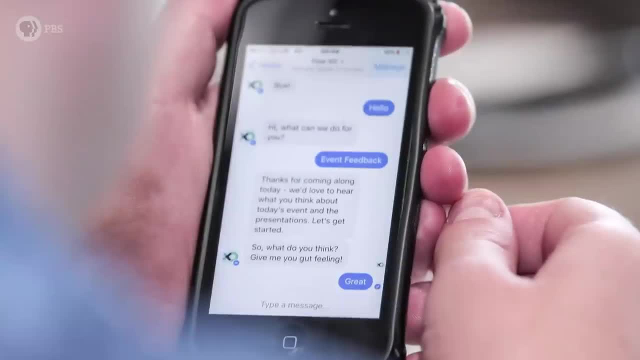 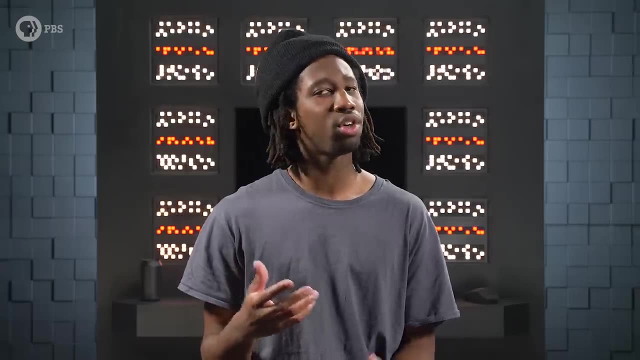 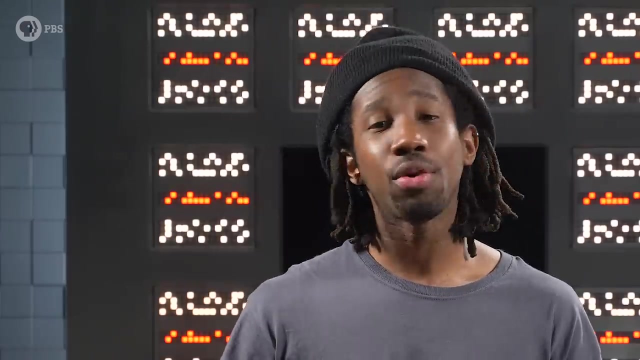 These are AI that perform translations, summarize documents or chat with you. The key to both problems is understanding the meaning of a word, which is tricky because words have no meaning on their own. We assign meaning to symbols To make things even harder. in many cases, language can be ambiguous and the meaning 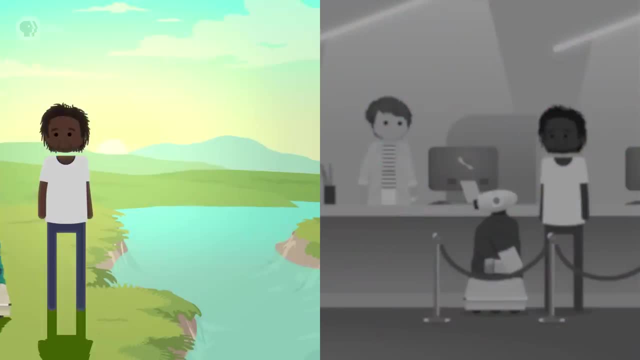 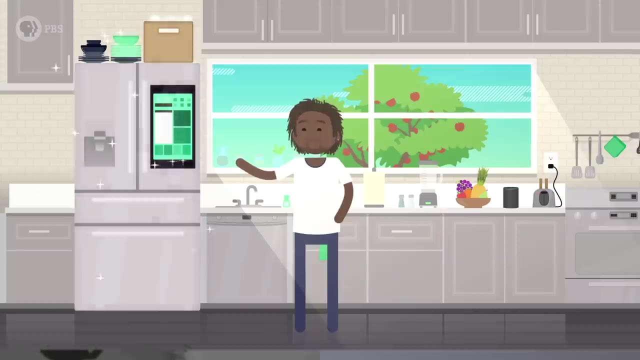 of a word depends on the language. It depends on the context it's used in. If I tell you to meet me at the bank, without context, I could mean the river bank or the place where I'm grabbing some cash. If I say this fridge is great, that's a totally different meaning from this fridge. 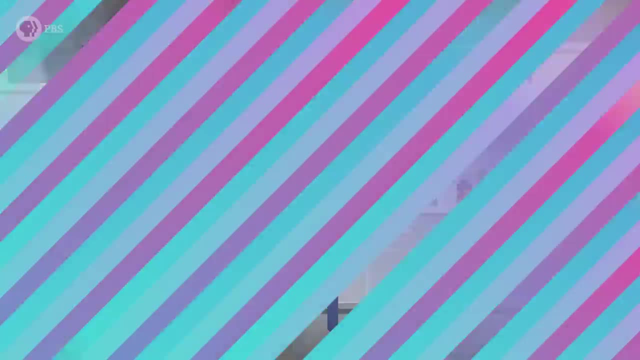 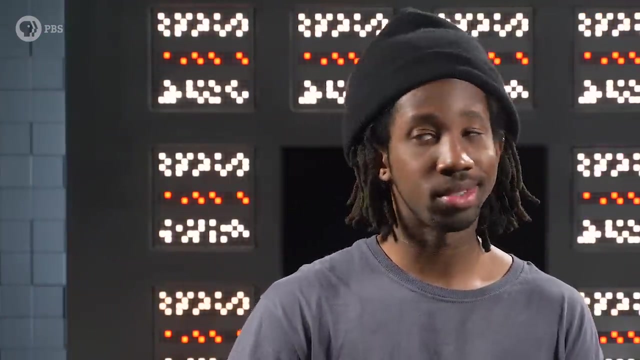 is great. It lasted a whole week before breaking. So how do we learn to attach meaning to sounds? How do we know great means something totally different from great? Well, even though there's nothing inherent in the word cat that tells us that it's. 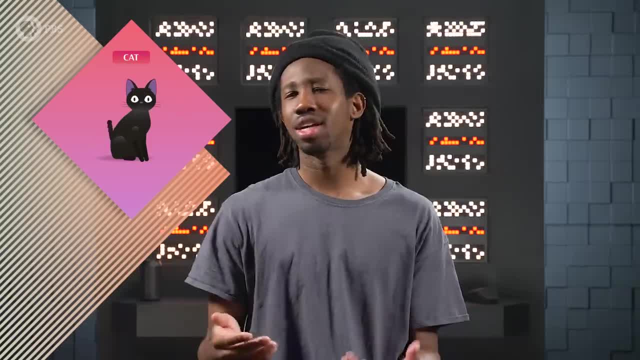 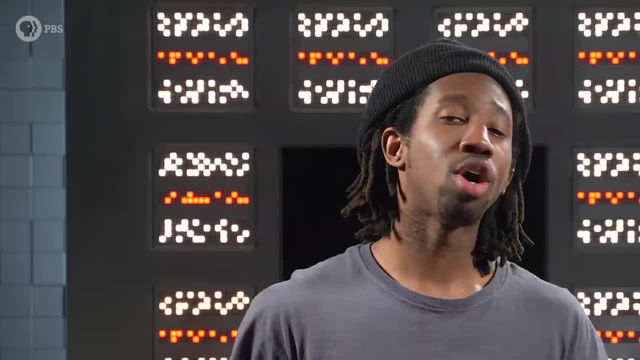 soft, purrs and chases mice. when we were kids, someone probably told us that this is a cat or a gato, maul, billy or ot. When we're solving a natural language processing problem, whether it's natural language understanding, 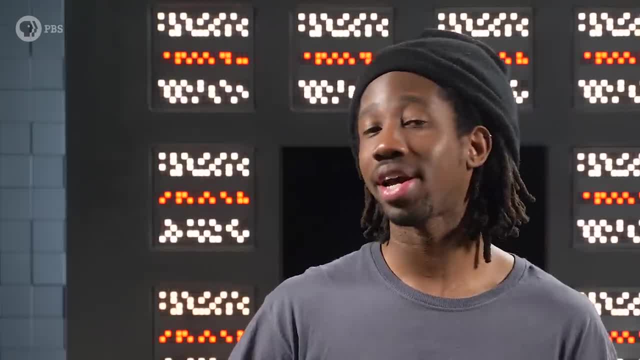 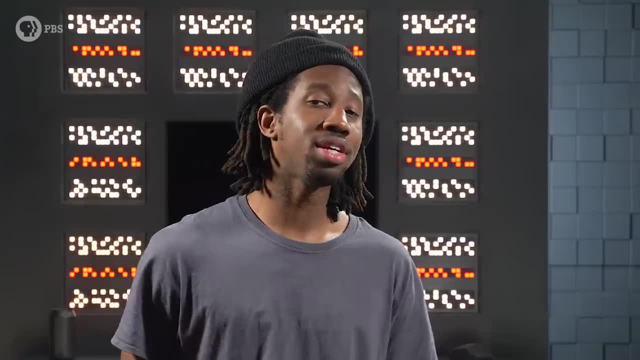 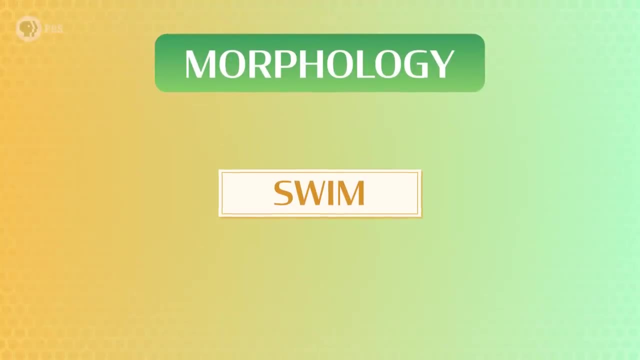 or natural language generation. we have to think about how our AI is going to learn the meaning of words and understand our potential mistakes. Sometimes we can compare words by looking at the letters they share. This works well if a word has morphology. Take the root word swim, for example. We can modify it with rules. So if someone's doing, 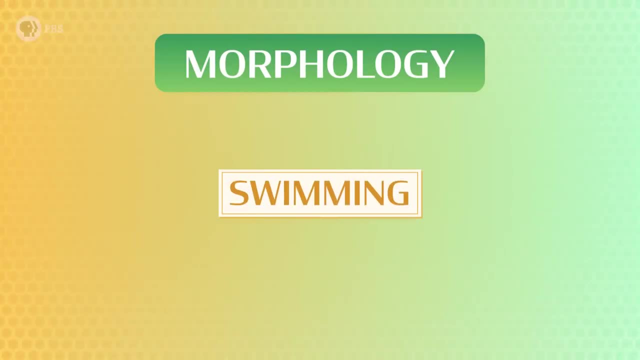 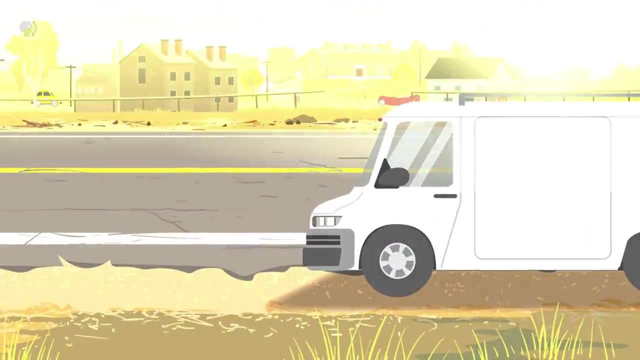 it. right now they're swimming, Or the person doing the action is the swimmer, Drinking, drinker, thinking, thinker. you get the idea, But we can't use morphology for all words Like how knowing that a van is a vehicle doesn't. 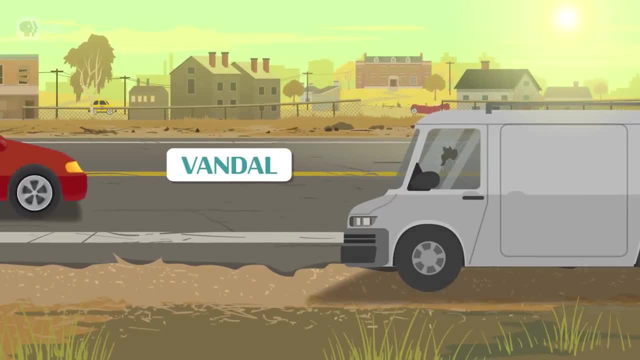 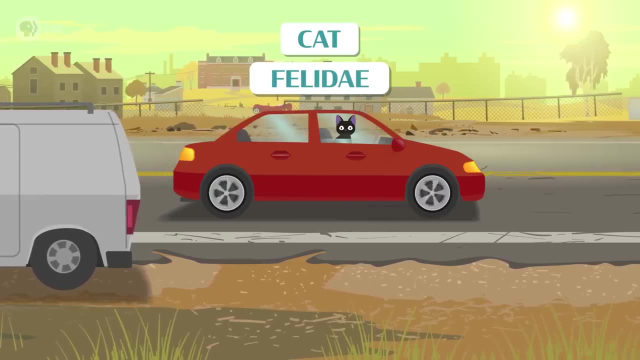 let us know that a vandal smashed in a window. Many words that are really similar, like cat and car, are completely unrelated, And cat and felidae, the word for the scientific family of cats, mean very similar things and only share one letter. 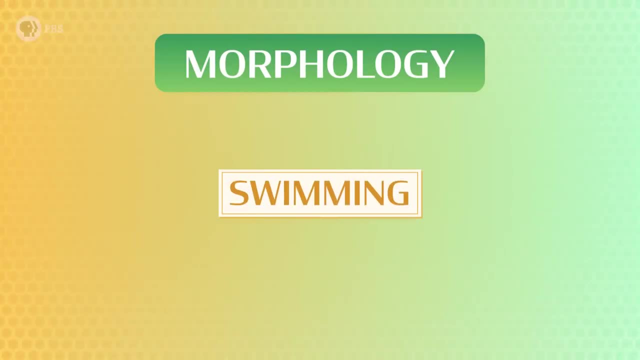 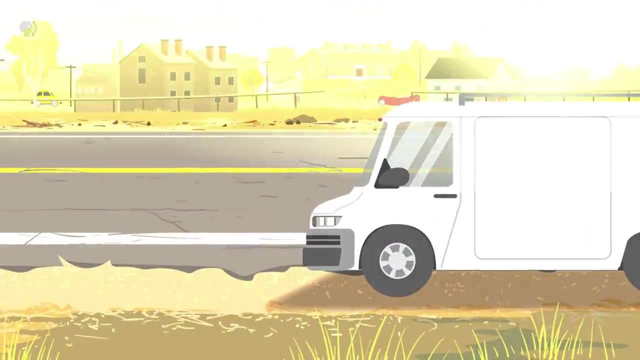 it. right now they're swimming, Or the person doing the action is the swimmer, Drinking, drinker, thinking, thinker. you get the idea, But we can't use morphology for all words Like how knowing that a van is a vehicle doesn't. 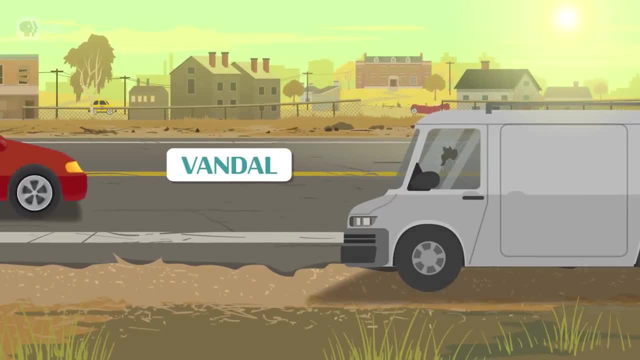 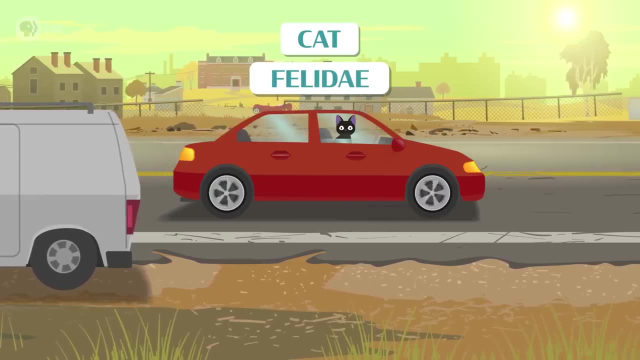 let us know that a vandal smashed in a window. Many words that are really similar, like cat and car, are completely unrelated, And cat and felidae, the word for the scientific family of cats, mean very similar things and only share one letter. 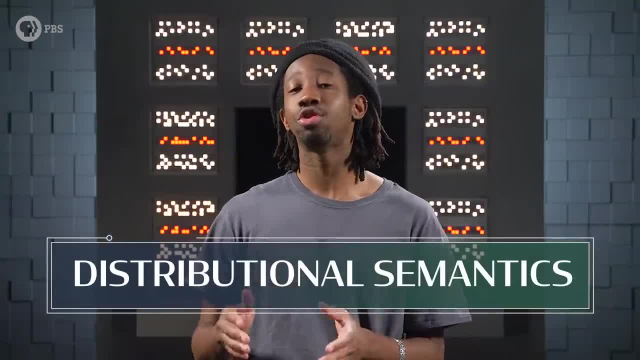 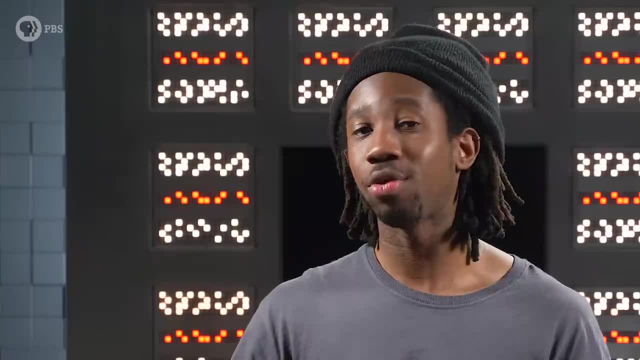 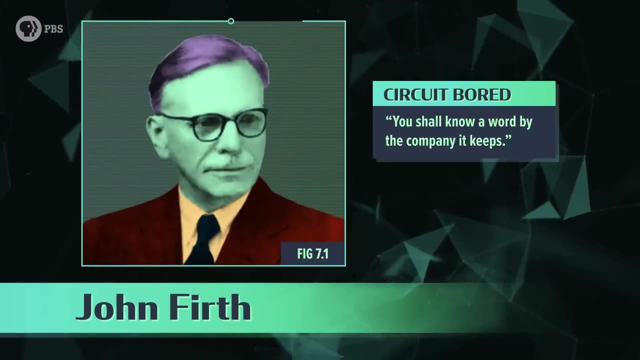 One common way to guess that words have similar meaning is using distributional semantics or seeing which words appear in the same sentences a lot. This is one of the many cases where NLP relies on insights from the field of linguistics. As the linguist John Firth once said, you shall know a word by the company it keeps. 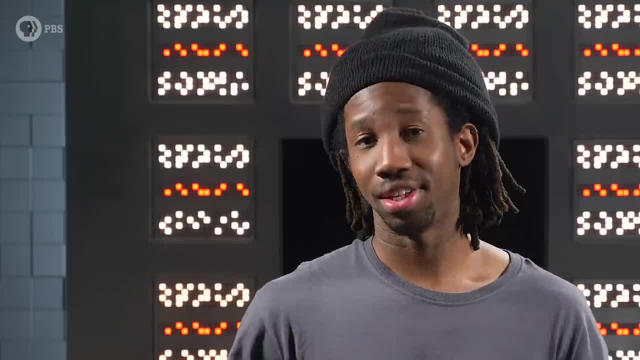 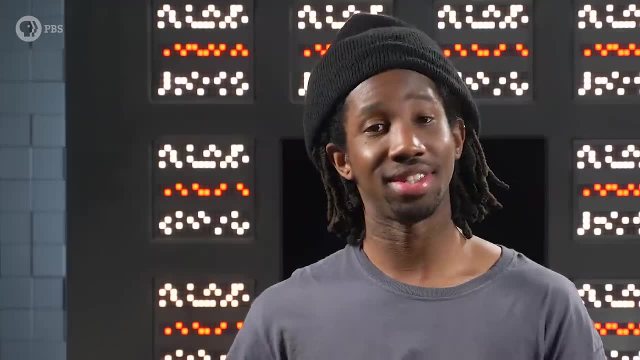 Instead, we have to express the concept in math. One simple technique is to use count vectors. A count vector is the number of times a word appears in the same article or sentence as other common words. If two words show up in the same sentence, they probably have pretty similar meanings. 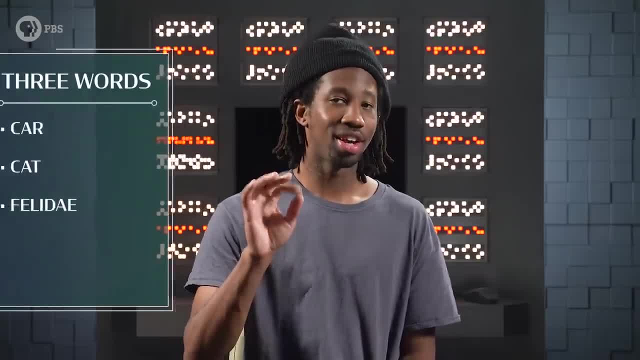 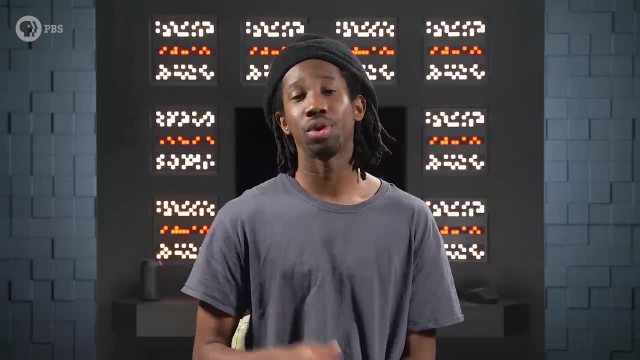 So let's say we asked an algorithm to compare three words- Car, cat and felidae- Using count vectors to guess which ones have similar meaning. We could download the beginning of the Wikipedia pages for each word which other words show up. 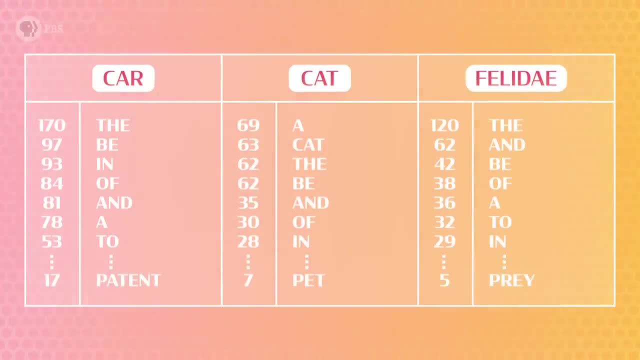 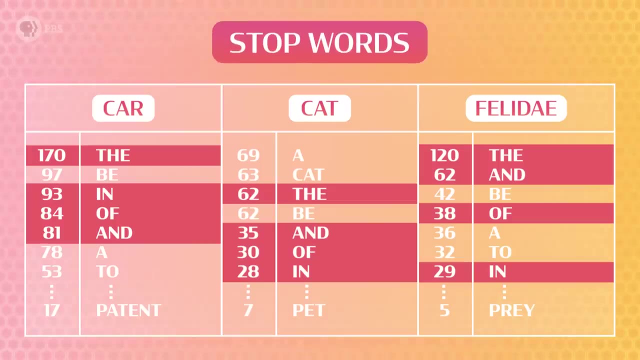 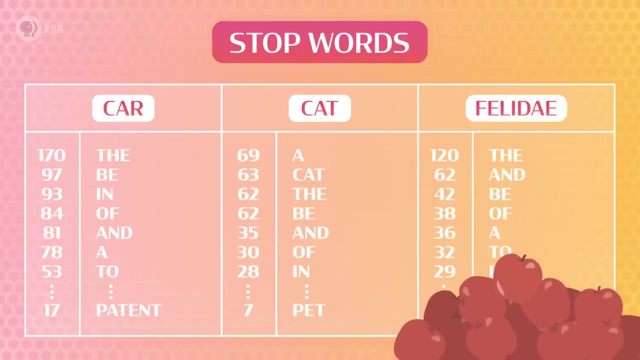 Here's what we got, And a lot of the top words are the same: the and of, in. These are all function words or stop words which help define the structure of language and help convey precise meaning, Like how an apple means any apple, but the apple specifies one in particular. 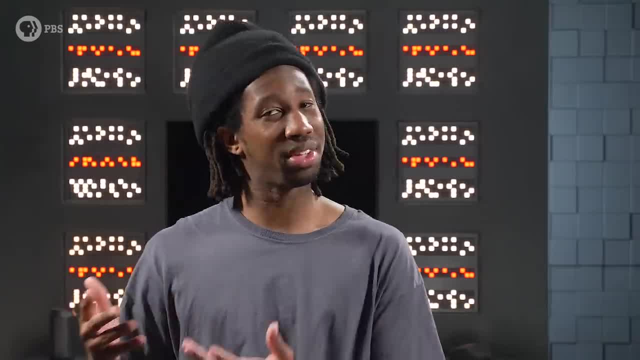 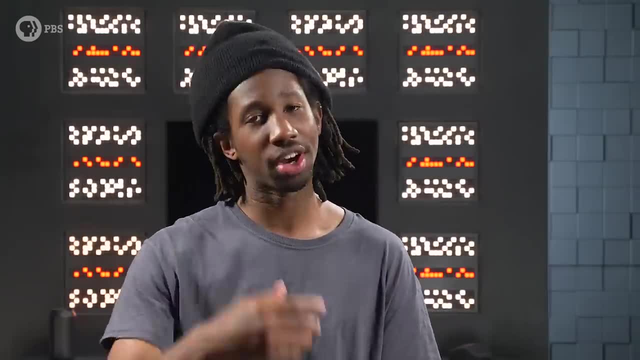 But because they change the meaning of other words. they don't have much meaning by themselves. So we'll remove them for now and simplify plurals and conjugations. Let's try it again. Based on this, it looks like cat and felidae mean almost the same thing, because they both. 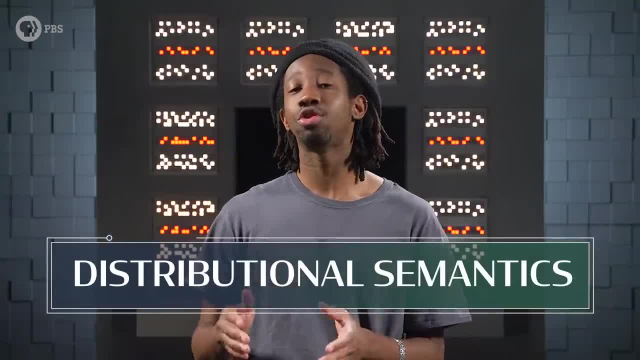 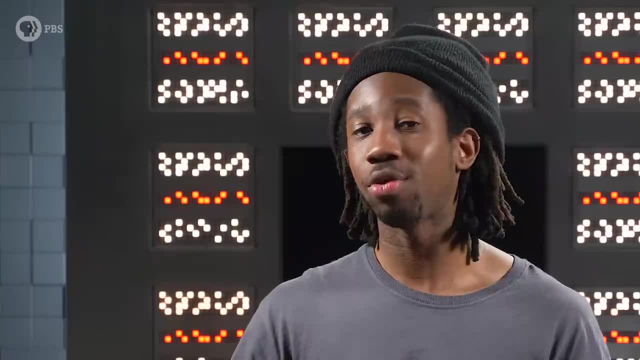 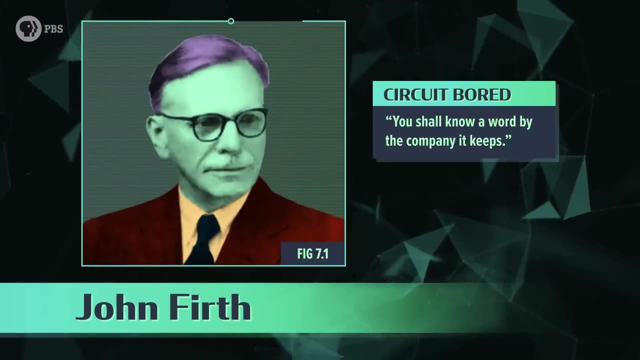 One common way to guess that words have similar meaning is using distributional semantics or seeing which words appear in the same sentences a lot. This is one of the many cases where NLP relies on insights from the field of linguistics. As the linguist John Firth once said, you shall know a word by the company it keeps. 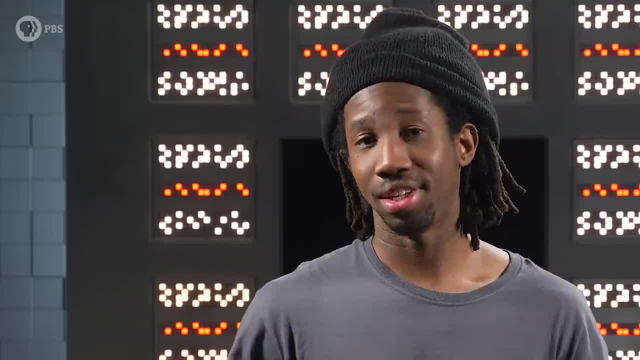 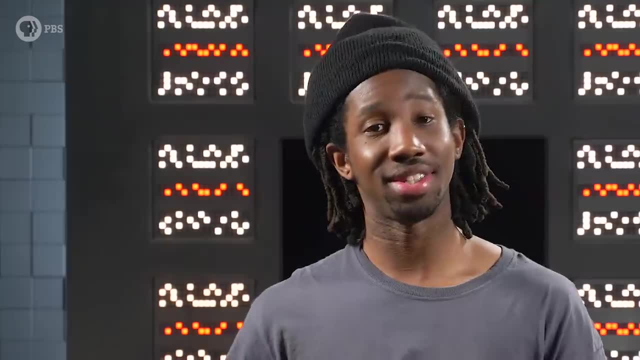 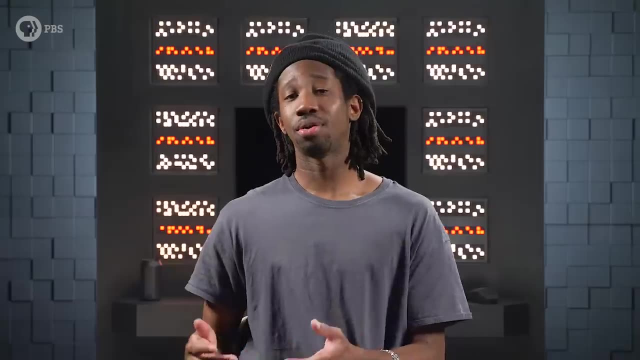 So it's definitely true. we have to express the concept in math. One simple technique is to use count vectors. A count vector is the number of times a word appears in the same article or sentence as other common words. If two words show up in the same sentence, they probably have pretty. 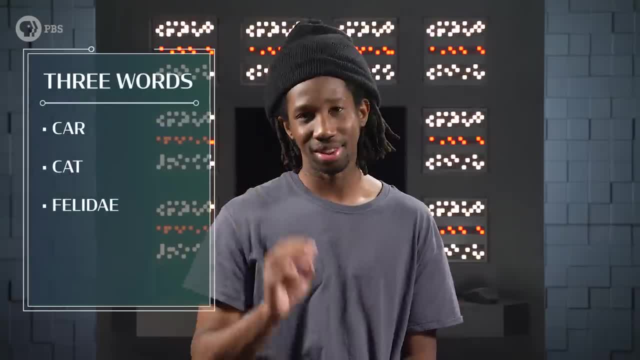 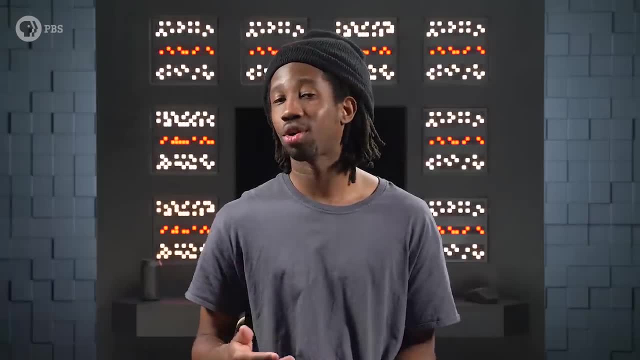 similar meanings. So let's say we asked an algorithm to compare three words- Car, cat and felidae- Using count vectors to guess which ones have similar meaning. We could download the beginning of the Wikipedia which other words show up. Here's what we got. 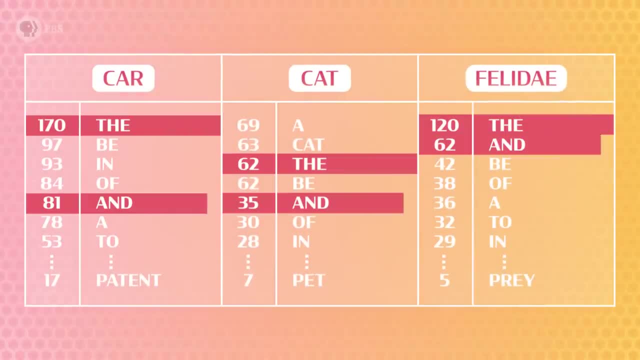 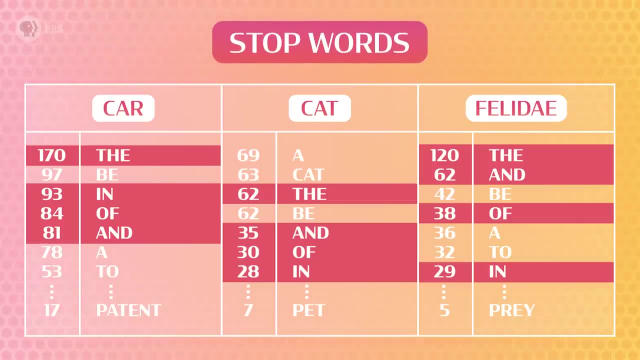 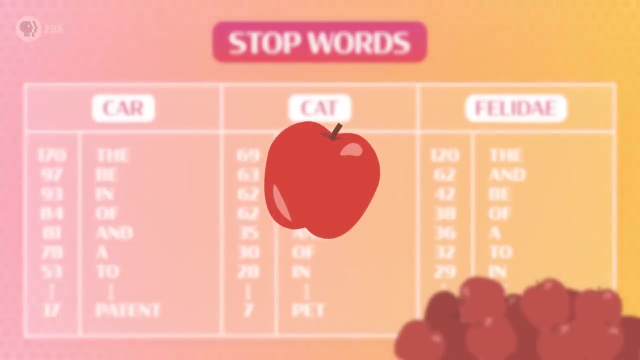 And a lot of the top words are the same: the and of, in. These are all function words or stop words which help define the structure of language and help convey precise meaning, Like how an apple means any apple, but the apple specifies one in particular. 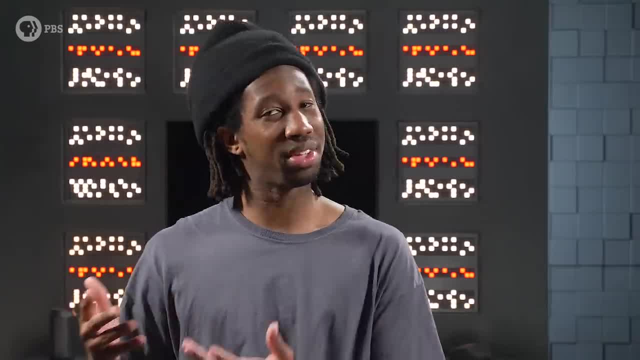 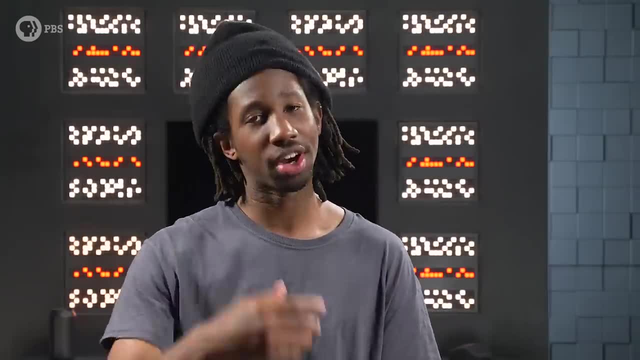 But because they change the meaning of other words. they don't have much meaning by themselves. So we'll remove them for now and simplify plurals and conjugations. Let's try it again. Based on this, it looks like cat and felidae mean almost the same thing, because they both. 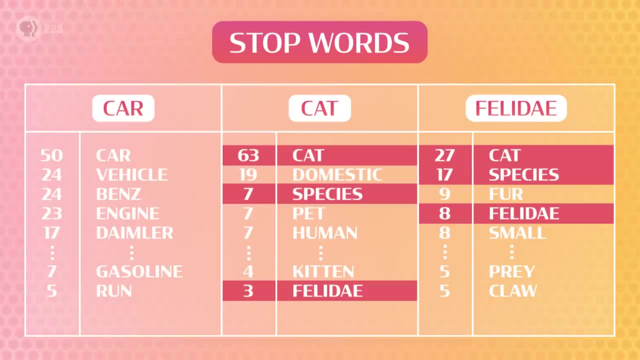 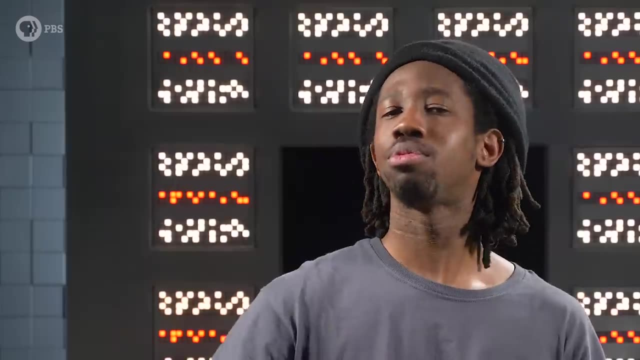 show up with lots of the same words in their Wikipedia articles, And neither of them mean the same thing as car. But this is also a really simplified example. One of the problems with count vectors is that we have to store a lot of data. 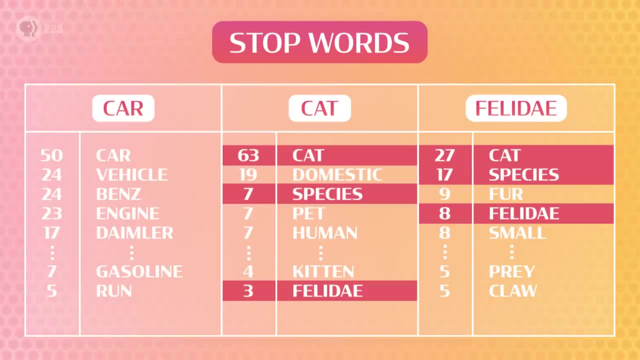 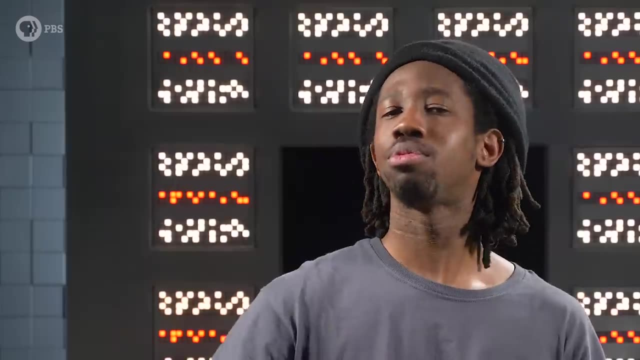 show up with lots of the same words in their Wikipedia articles, And neither of them mean the same thing as car. But this is also a really simplified example. One of the problems with count vectors is that we have to store a lot of data. 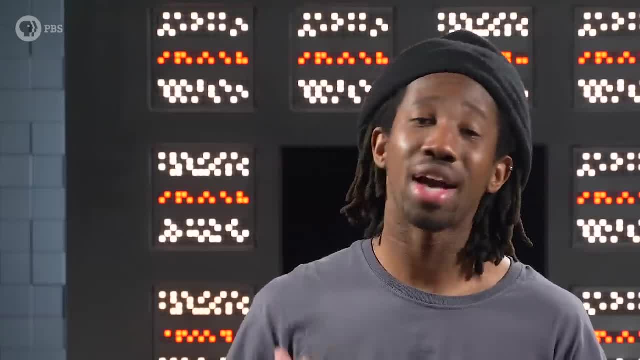 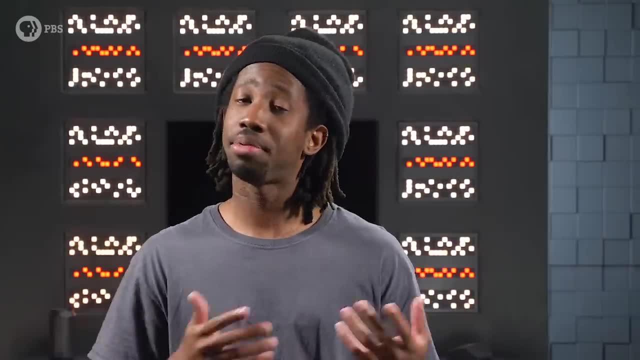 To compare a bunch of words using count vectors like this. we'd need a massive list of every word we've ever seen in the same sentence, And that's unmanageable, So we'd like to learn a representation for words that captures all the same relationships. 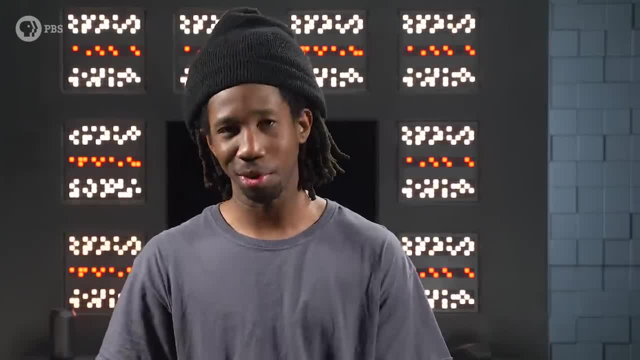 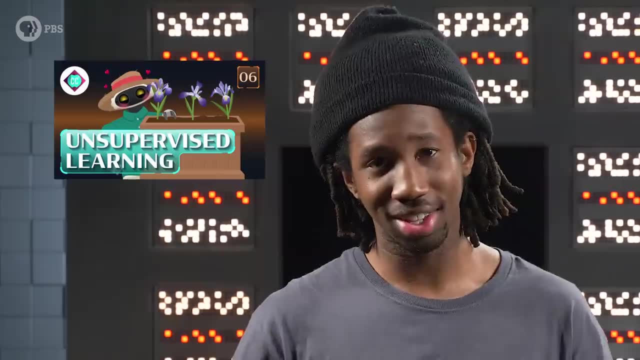 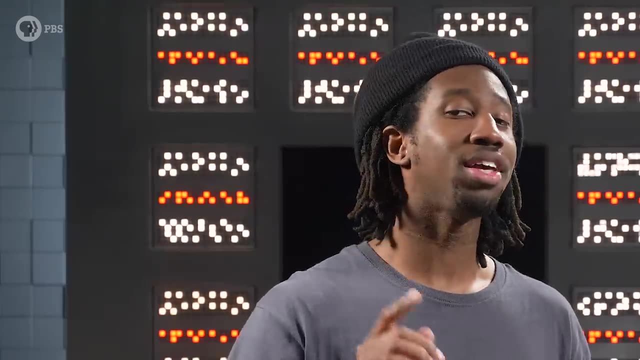 and similarities as count vectors, but is much more compact. In the unsupervised learning episode, we talked about how to compare images by building representations of those images. We needed a model that could build internal representations and that could generate predictions. We can do the same thing for words. 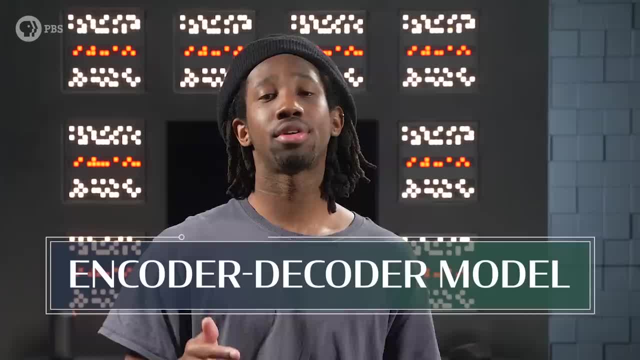 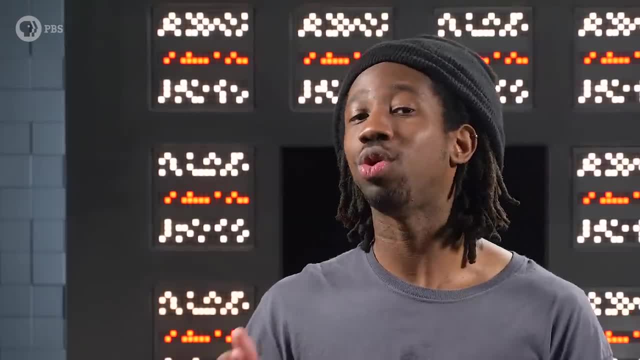 This is called an encoder diagram. It's a decoder model. The encoder tells us what we should think and remember about what we just read, And the decoder uses that thought to decide what we want to say or do. We're going to start with a simple version of this framework. 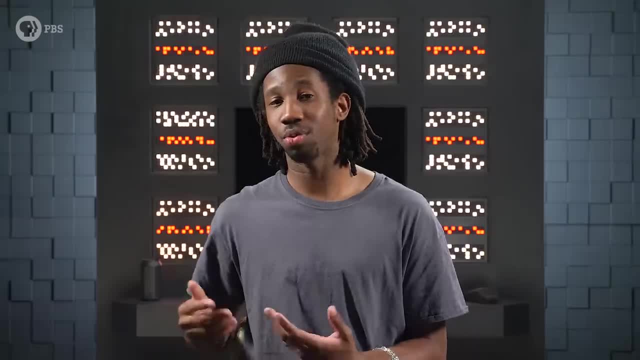 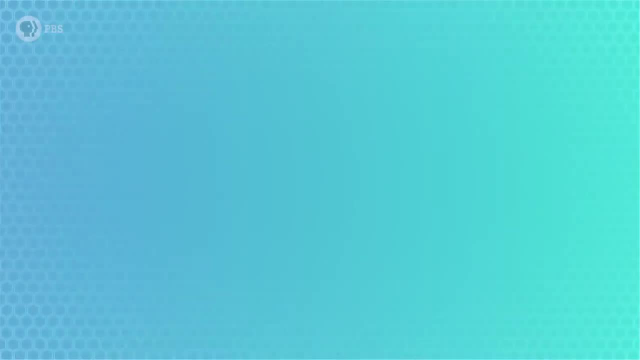 Let's create a little game of fill in the blank to see what basic pieces we need to train an unsupervised learning model. This is a simple task called language modeling. If I have the sentence, I'm kind of hungry. I think I'd like some chocolate ________. 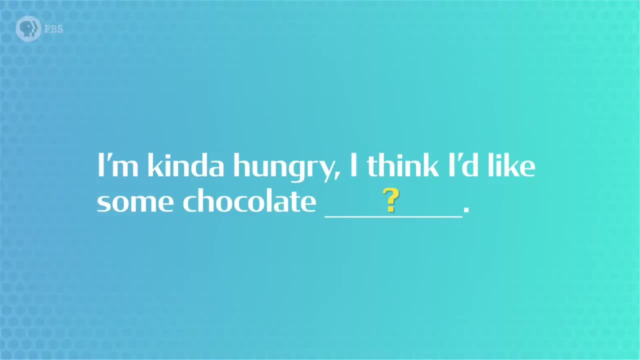 What are the most likely words That can go in that spot And how might we train a model to encode the sentence and decode a guess for the blank In this example? I can guess the answer might be cake or milk, but probably not something. 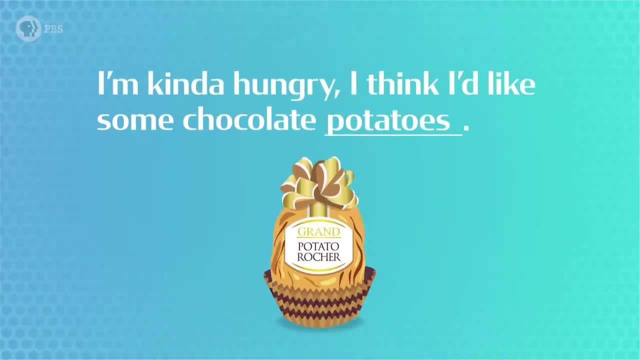 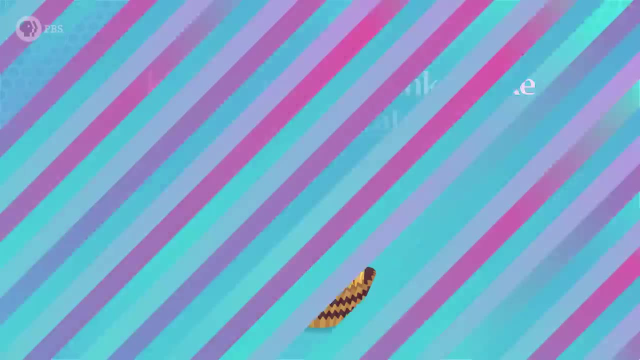 like potatoes, because I've never heard of chocolate potatoes, so they probably don't exist, Definitely don't exist. That should not be a thing. The group of words that can fill in that blank is an unsupervised cluster that an AI could. 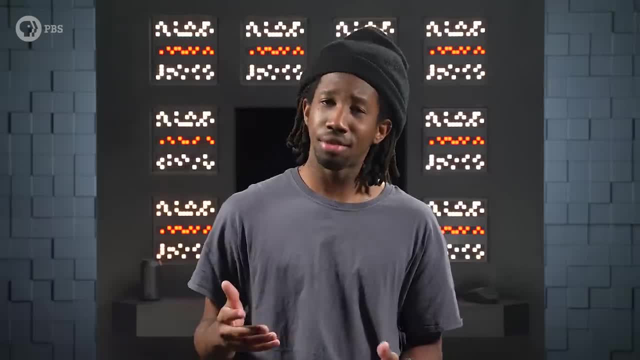 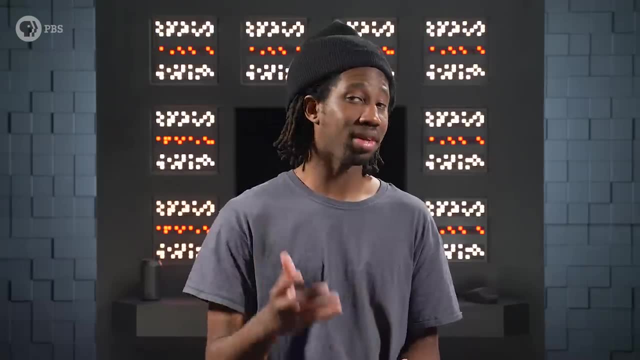 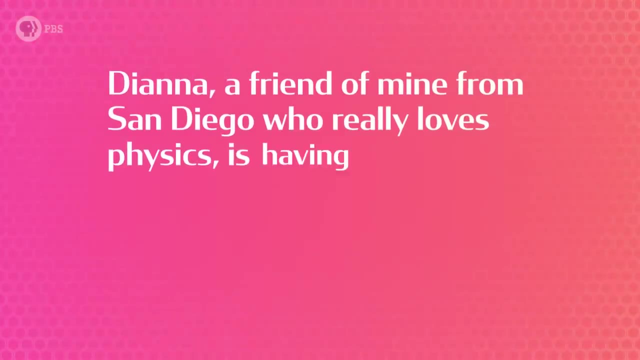 use. So for this sentence our encoder might only need to focus on the word chocolate, so the decoder has a cluster of chocolate food words to pull from to fill in that blank. Now let's try a harder example. Diana, a friend of mine from San Diego who really loves physics, is having a birthday. 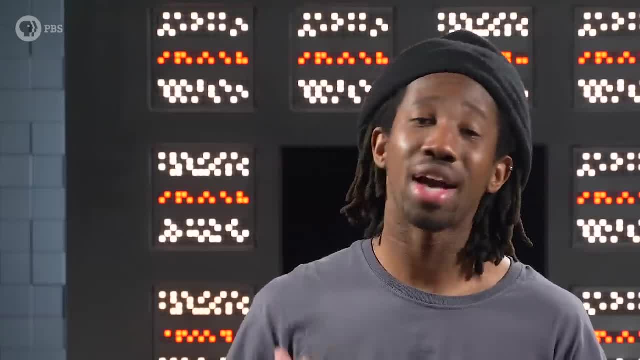 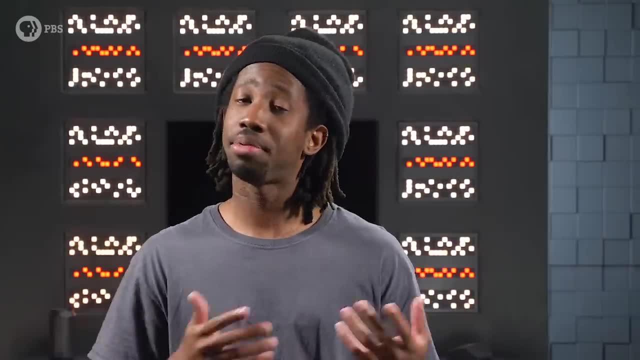 To compare a bunch of words using count vectors like this. we'd need a massive list of every word we've ever seen in the same sentence, And that's unmanageable, So we'd like to learn a representation for words that captures all the same relationships. 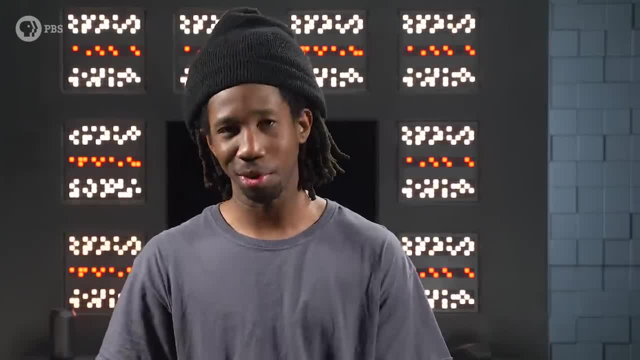 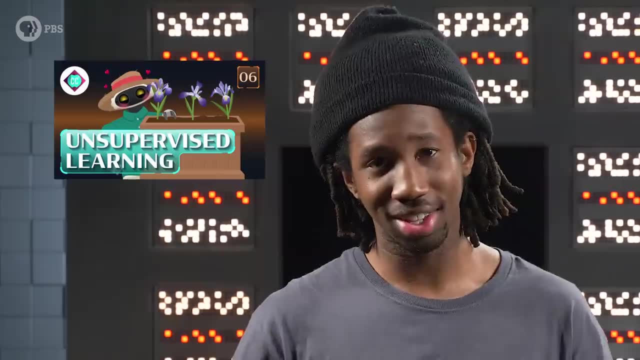 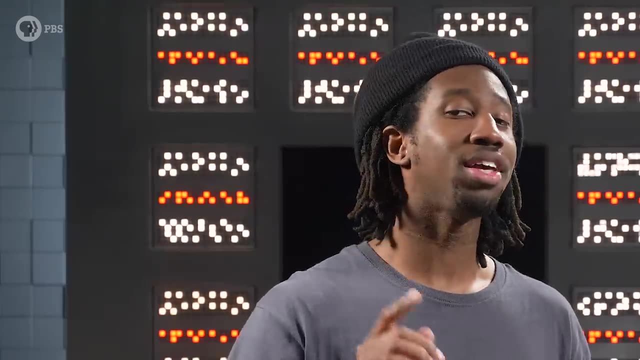 and similarities as count vectors, but is much more compact. In the unsupervised learning episode, we talked about how to compare images by building representations of those images. We needed a model that could build internal representations and that could generate predictions. We can do the same thing for words. 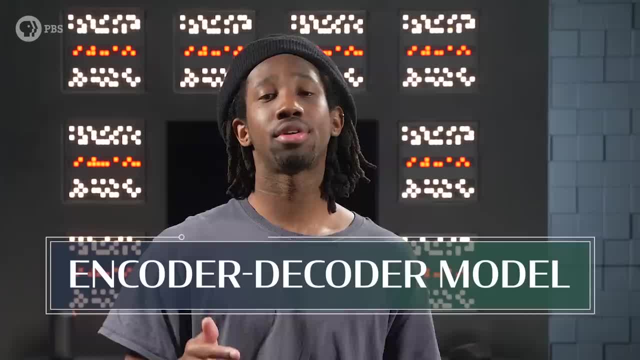 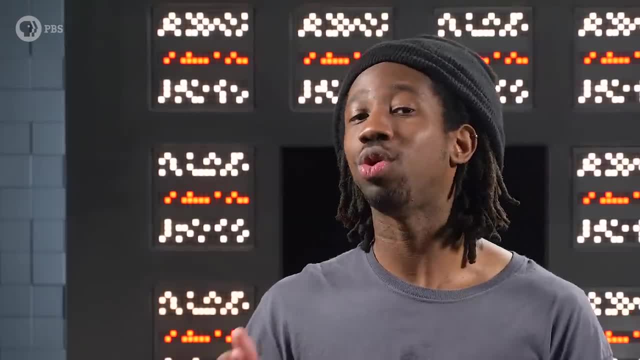 This is called an encoder diagram. It's a decoder model. The encoder tells us what we should think and remember about what we just read, And the decoder uses that thought to decide what we want to say or do. We're going to start with a simple version of this framework. 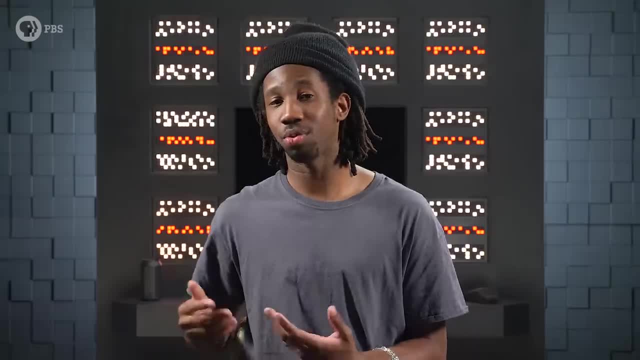 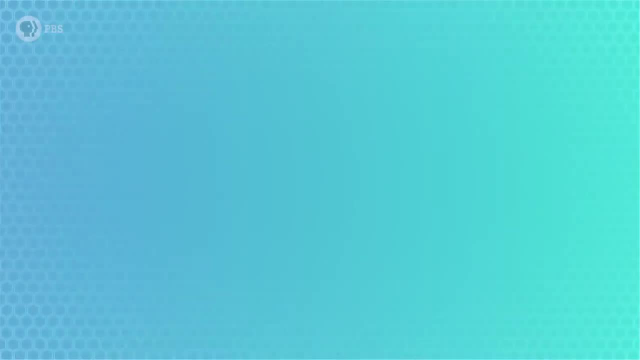 Let's create a little game of fill in the blank to see what basic pieces we need to train an unsupervised learning model. This is a simple task called language modeling. If I have the sentence, I'm kind of hungry. I think I'd like some chocolate ________. 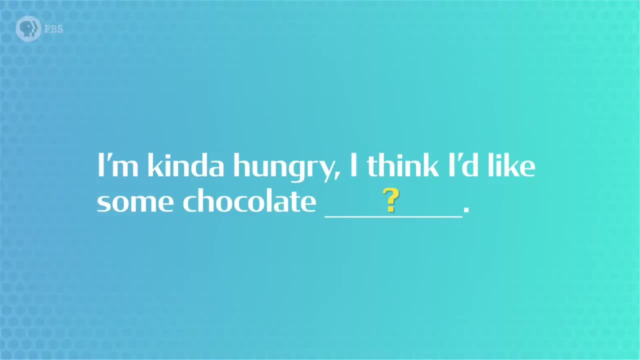 What are the most likely words That can go in that spot And how might we train a model to encode the sentence and decode a guess for the blank In this example? I can guess the answer might be cake or milk, but probably not something. 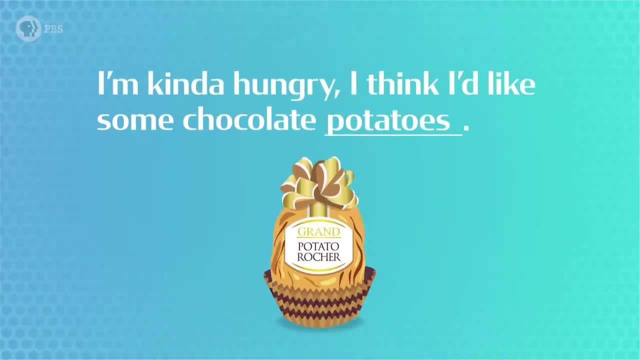 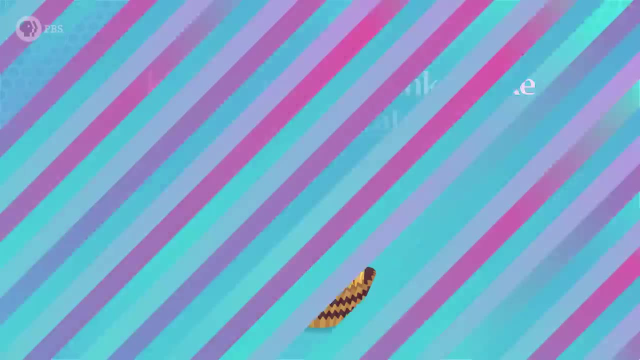 like potatoes, because I've never heard of chocolate potatoes, so they probably don't exist, Definitely don't exist. That should not be a thing. The group of words that can fill in that blank is an unsupervised cluster that an AI could. 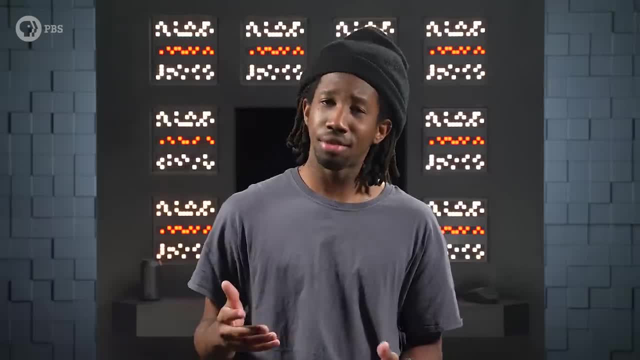 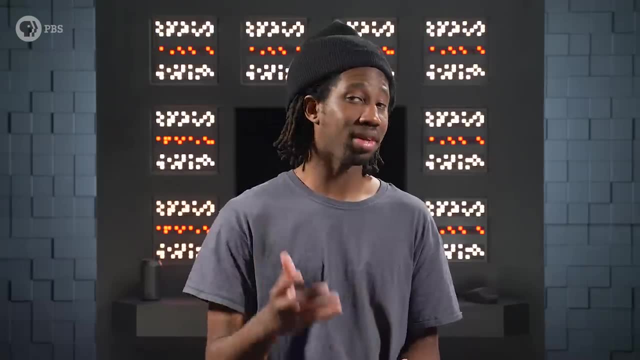 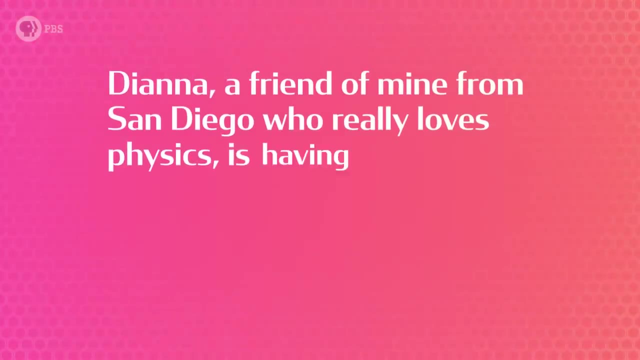 use. So for this sentence our encoder might only need to focus on the word chocolate, so the decoder has a cluster of chocolate food words to pull from to fill in that blank. Now let's try a harder example. Diana, a friend of mine from San Diego who really loves physics, is having a birthday. 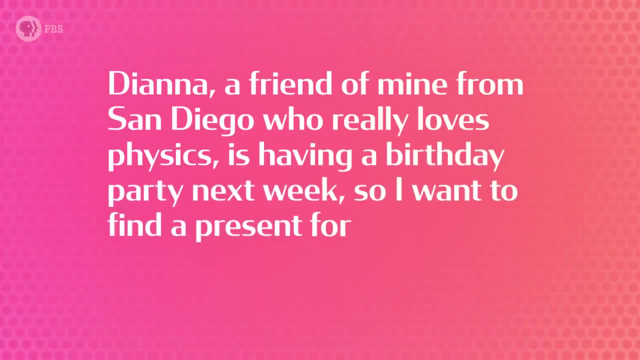 party next week, so I want to find a present for ________. When I read this sentence, my brain identifies and remembers two things: First, that we're talking about Diana from 27 words ago And second, that my friend Diana uses the pronoun her. 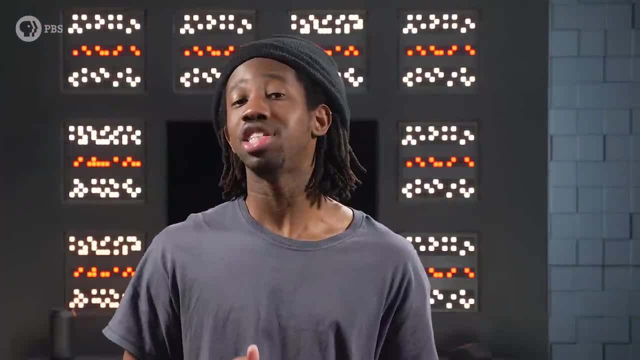 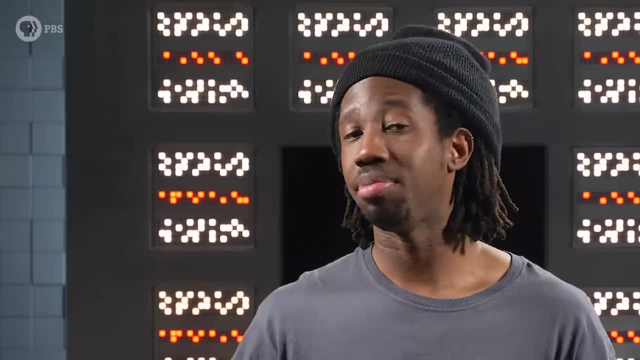 That means we want our encoder to build a representation that captures all these pieces of information from the sentence so that the decoder can choose the right word for that blank. And if we keep the sentence going, Diana, a friend of mine from San Diego who really 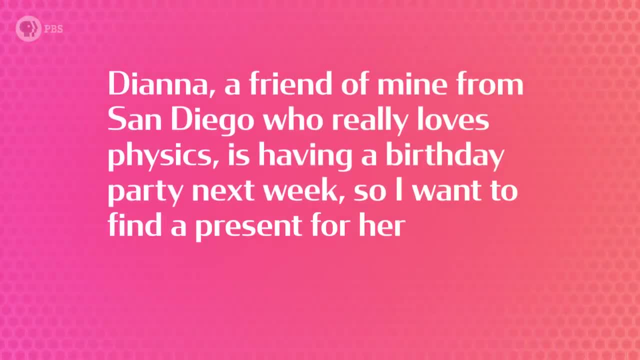 loves physics, is having a birthday party next week, so I want to find a present for her that has to do with ________. Now, I can remember that Diana likes physics from earlier in the sentence, So we'd like our decoder to choose the right word for that blank. 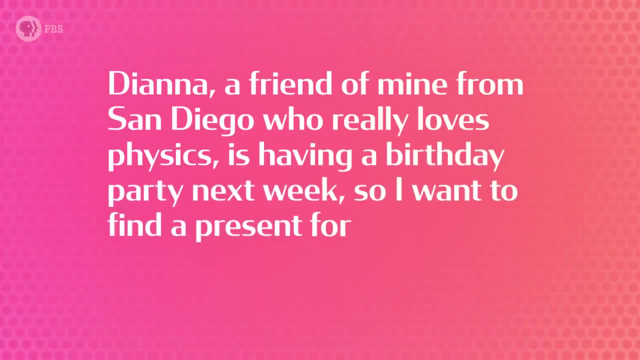 party next week, so I want to find a present for ________. When I read this sentence, my brain identifies and remembers two things: First, that we're talking about Diana from 27 words ago And second, that my friend Diana uses the pronoun her. 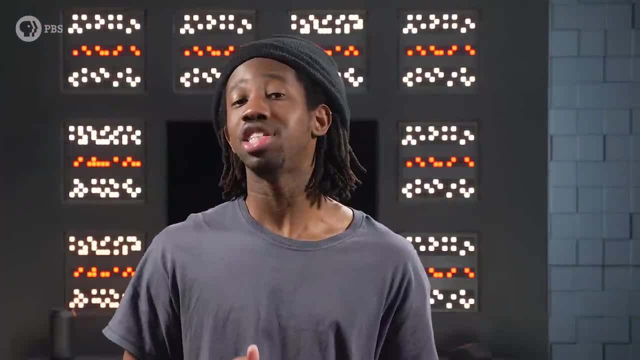 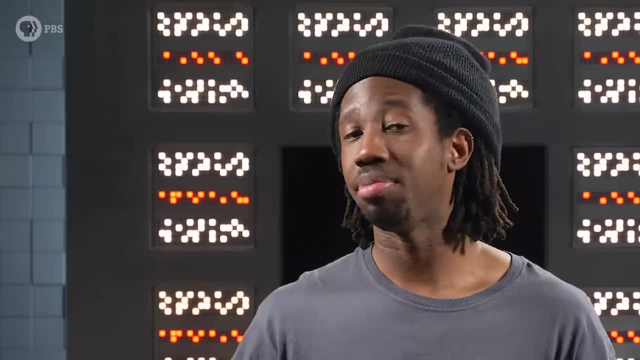 That means we want our encoder to build a representation that captures all these pieces of information from the sentence so that the decoder can choose the right word for that blank. And if we keep the sentence going, Diana, a friend of mine from San Diego who really 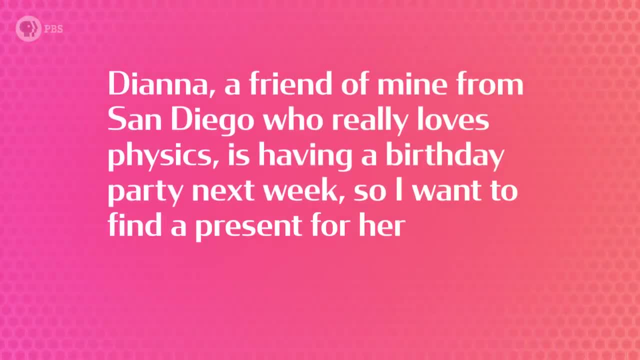 loves physics, is having a birthday party next week, so I want to find a present for her that has to do with ________. Now, I can remember that Diana likes physics from earlier in the sentence, So we'd like our decoder to choose the right word for that blank. 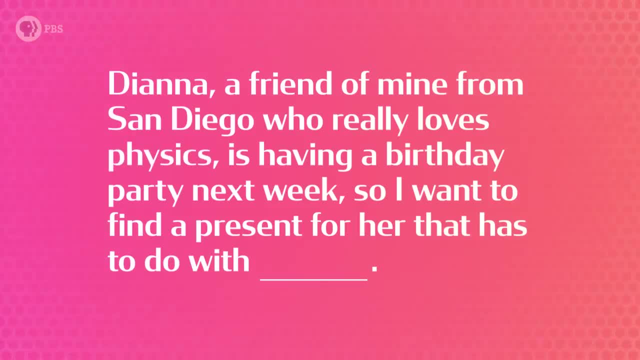 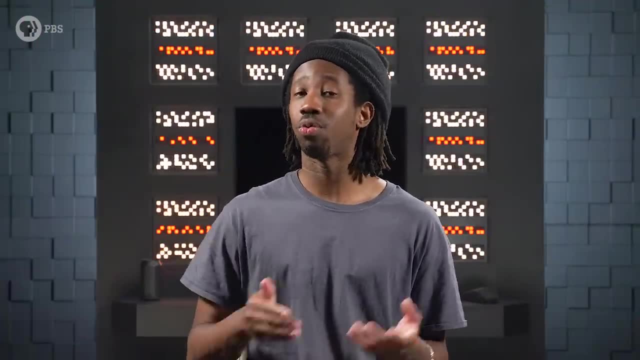 And we'd like our encoder to remember that too, so that the decoder can use that information to guess the answer. So we can see how the representation the model builds really has to remember key details of what we've said or heard. And there's a limit to how much a model can remember. 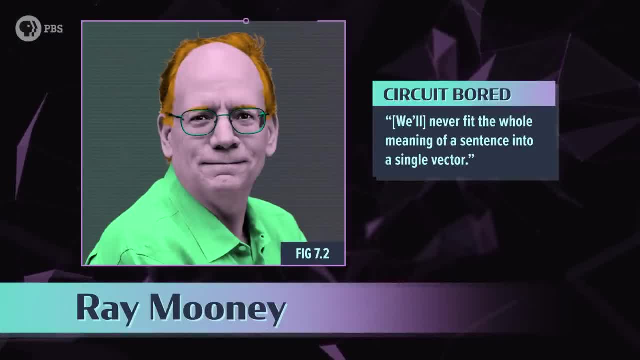 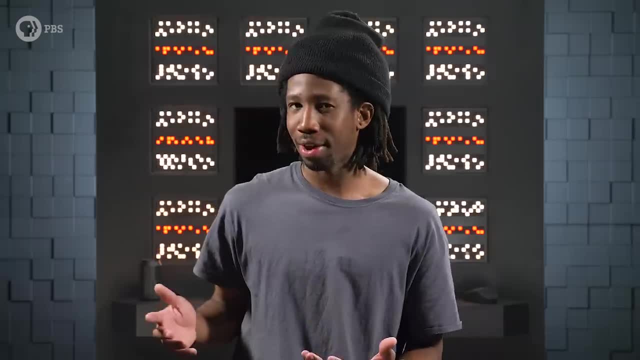 Professor Ray Mooney has famously said that we'll never fit the whole meaning of a sentence into a single vector, And we still don't know if we can. Professor Mooney may be right, but that doesn't mean we can't make something useful. 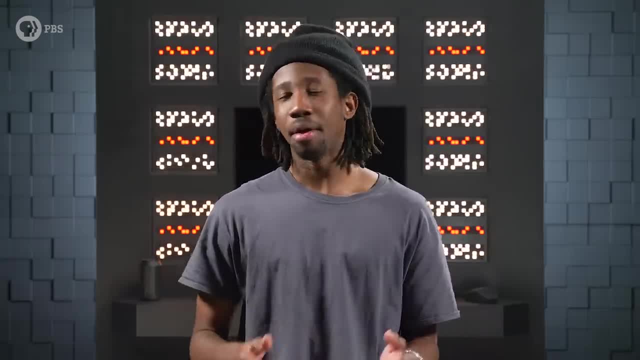 So far we've been using the verb to describe a sentence. So far we've been using the verb to describe a sentence. So far we've been using the verb to describe a sentence. We've been using words in our models, but computers don't work with words quite like. 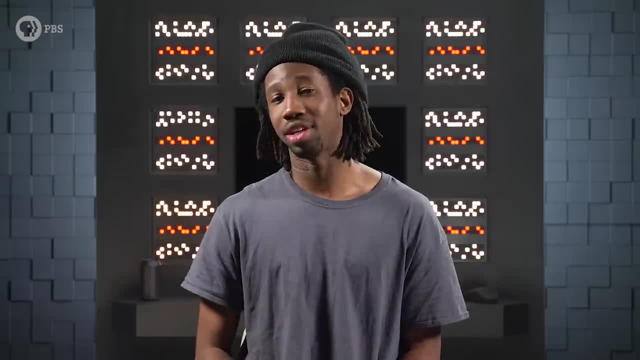 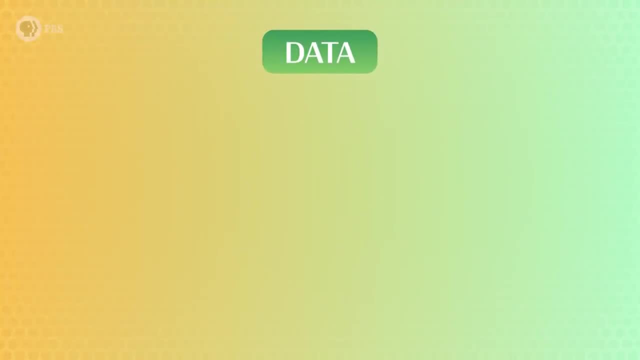 this. So let's step away from our high-level view of language modeling and try to predict the next word in a sentence using a neural network To do this. our data will be lots of sentences we collect from things like someone speaking. 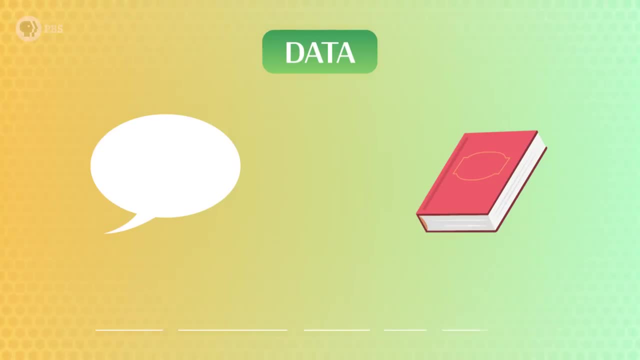 or text from books. Then for each word, in every sentence, we'll play a game of fill in the blank. We'll train a model to encode up to that blank and then predict the word that should go there. And since we have the whole sentence, we know the correct answer. 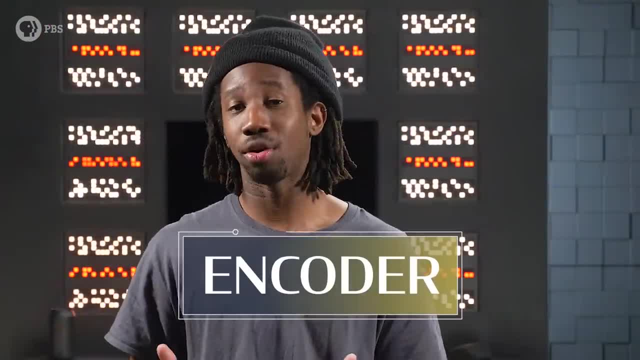 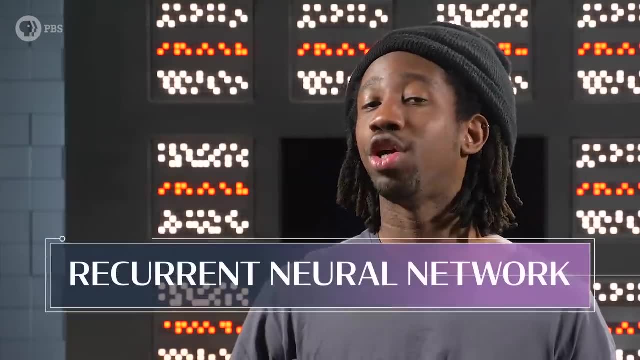 First, we need to define the encoder. We need a model that can read in the input, which in this case is a sentence. To do this, we'll use a type of neural network called a recurrent neural network or RNN. 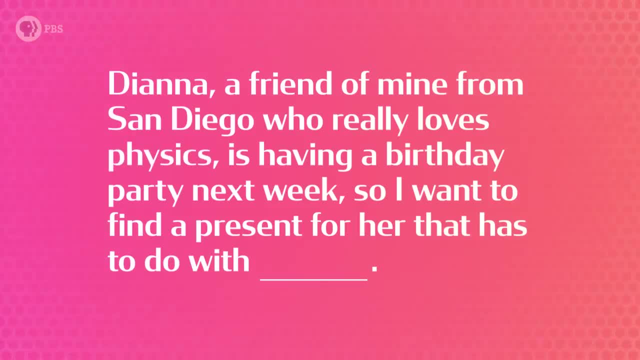 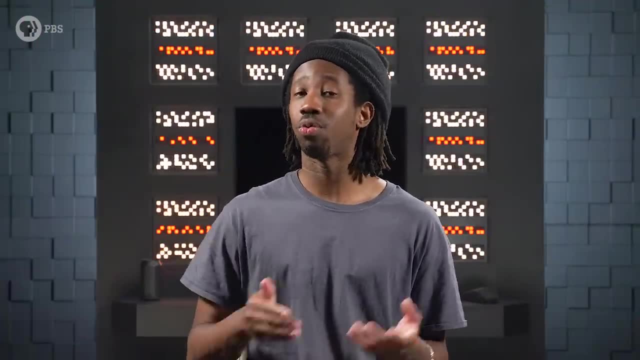 And we'd like our encoder to remember that too, so that the decoder can use that information to guess the answer. So we can see how the representation the model builds really has to remember key details of what we've said or heard. And there's a limit to how much a model can remember. 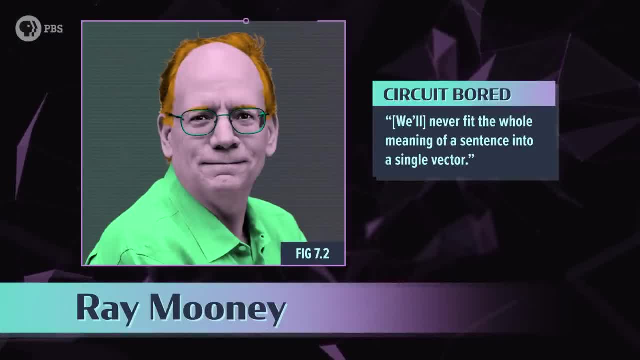 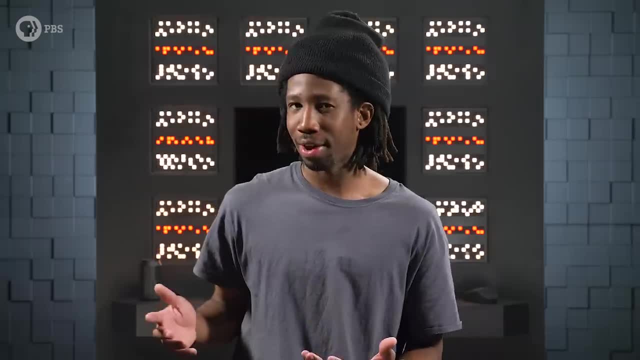 Professor Ray Mooney has famously said that we'll never fit the whole meaning of a sentence into a single vector, And we still don't know if we can. Professor Mooney may be right, but that doesn't mean we can't make something useful. 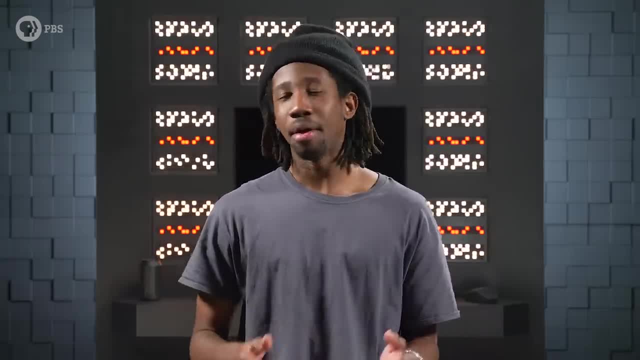 So far we've been using the verb to describe a sentence. So far we've been using the verb to describe a sentence. So far we've been using the verb to describe a sentence. We've been using words in our models, but computers don't work with words quite like. 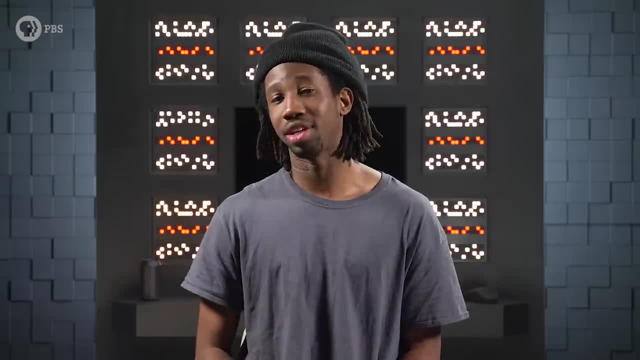 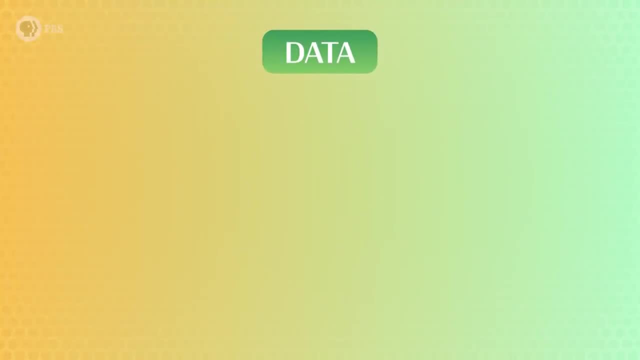 this. So let's step away from our high-level view of language modeling and try to predict the next word in a sentence using a neural network To do this. our data will be lots of sentences we collect from things like someone speaking. 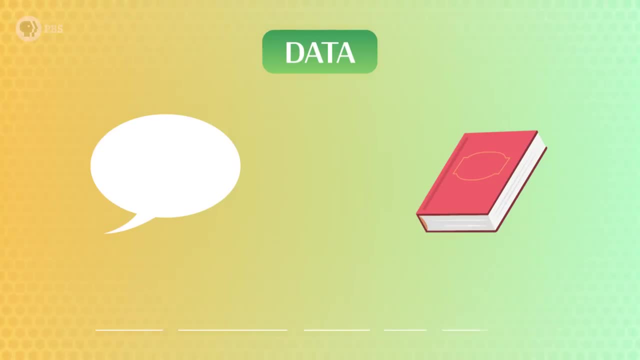 or text from books. Then for each word, in every sentence, we'll play a game of fill in the blank. We'll train a model to encode up to that blank and then predict the word that should go there. And since we have the whole sentence, we know the correct answer. 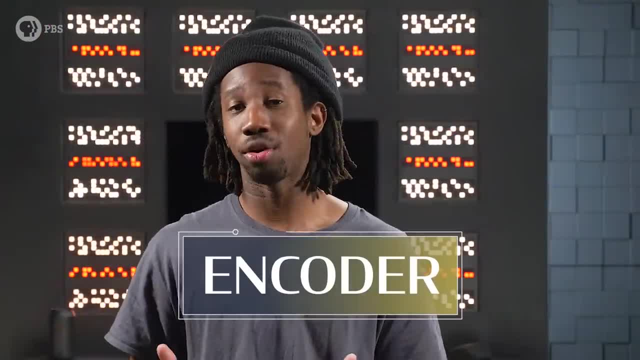 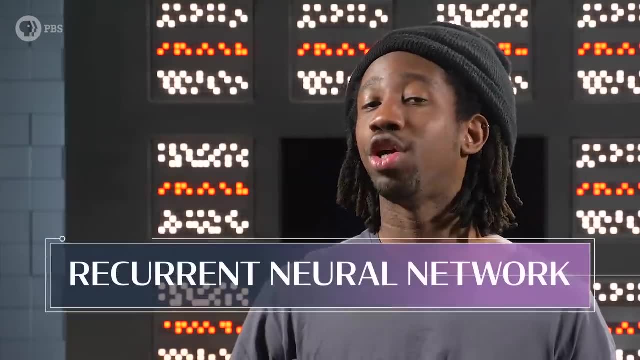 First, we need to define the encoder. We need a model that can read in the input, which in this case is a sentence. To do this, we'll use a type of neural network called a recurrent neural network or RNN. 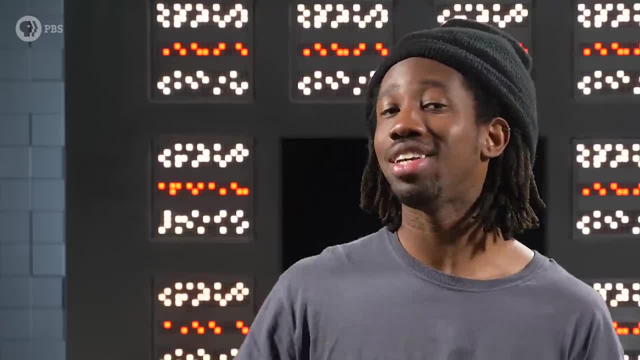 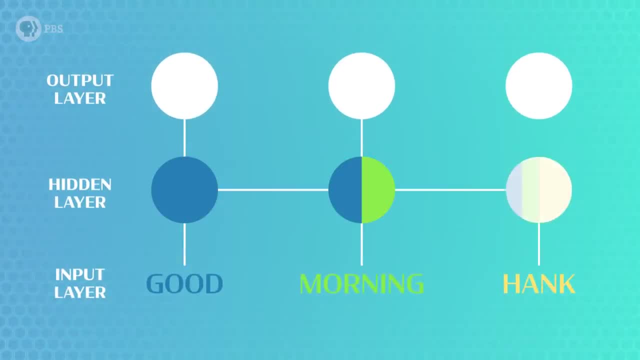 for short, RNNs have a loop in them that lets them reuse a single hidden layer which gets updated as the model reads one word at a time. Slowly, the model builds up an understanding of the whole sentence, including which words came first or last, which words are modifying other words and a whole bunch of other grammatical. 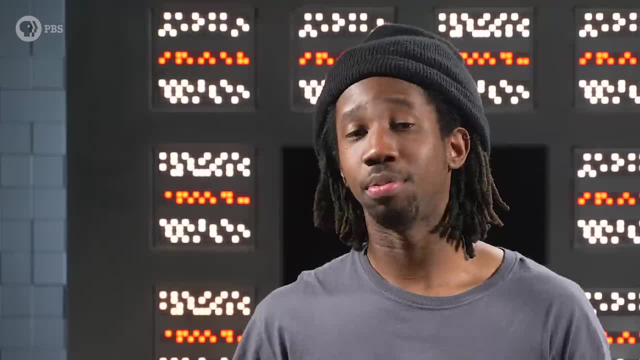 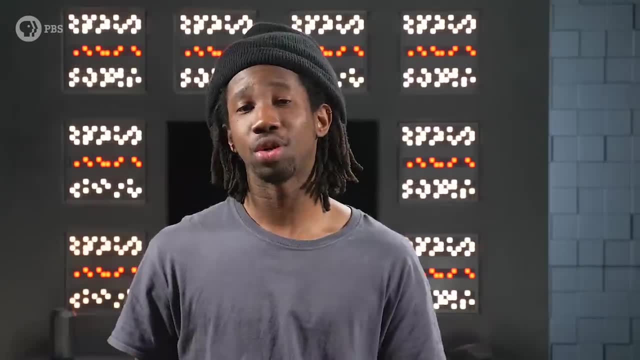 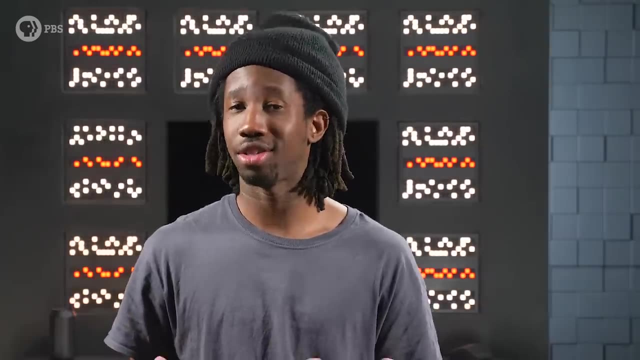 properties that are linked to meaning. Now, we can't just directly put words inside a network, but we also don't have features we can easily measure and give the model either. Unlike images, we can't even measure pixel values, So we're going to ask the model to learn the right representation for a word on its 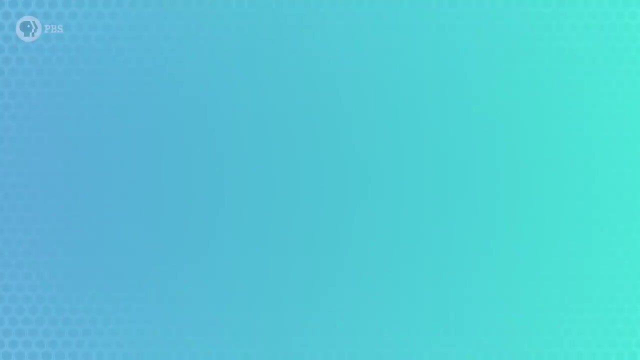 own. This is where unsupervised learning comes in. To do this, we'll start off by assigning each word a random representation, In this case a random list of numbers called a vector. Next, our encoder will take in each of those representations and combine them into a single. 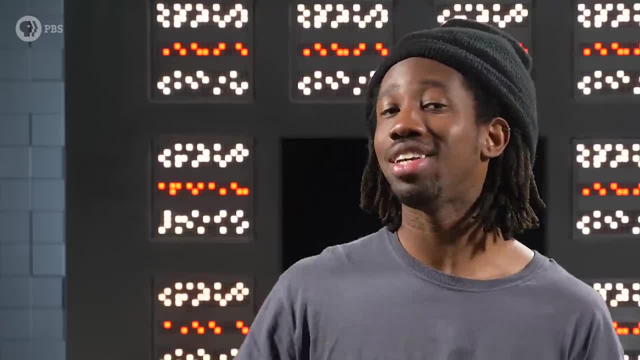 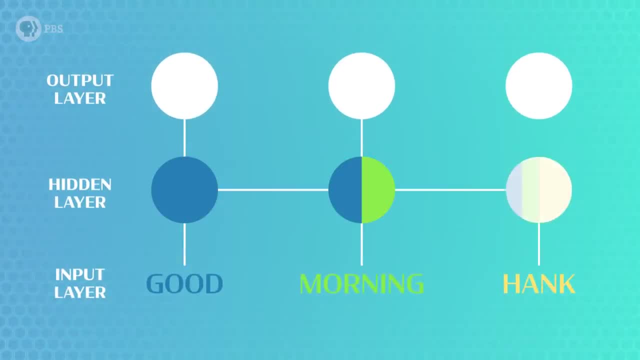 for short, RNNs have a loop in them that lets them reuse a single hidden layer which gets updated as the model reads one word at a time. Slowly, the model builds up an understanding of the whole sentence, including which words came first or last, which words are modifying other words and a whole bunch of other grammatical. 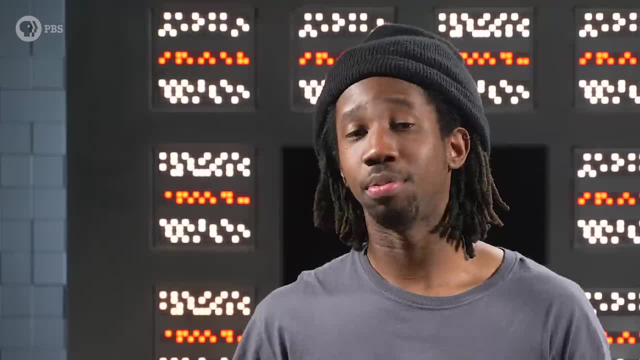 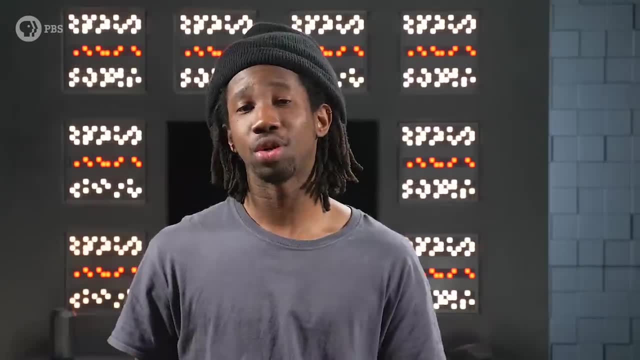 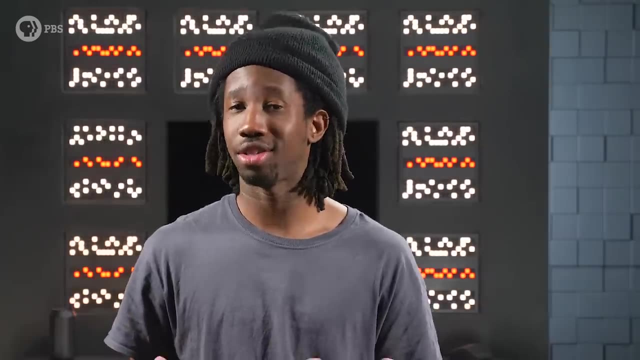 properties that are linked to meaning. Now, we can't just directly put words inside a network, but we also don't have features we can easily measure and give the model either. Unlike images, we can't even measure pixel values, So we're going to ask the model to learn the right representation for a word on its 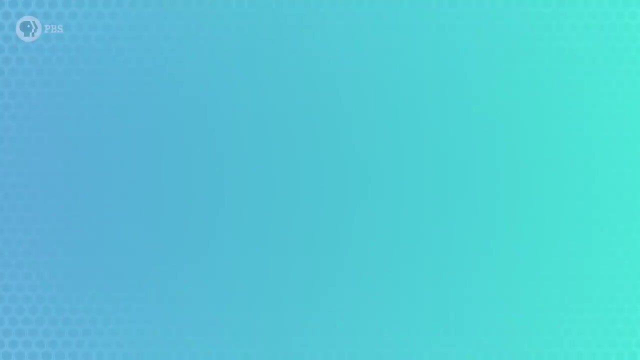 own. This is where unsupervised learning comes in. To do this, we'll start off by assigning each word a random representation, In this case a random list of numbers called a vector. Next, our encoder will take in each of those representations and combine them into a single. 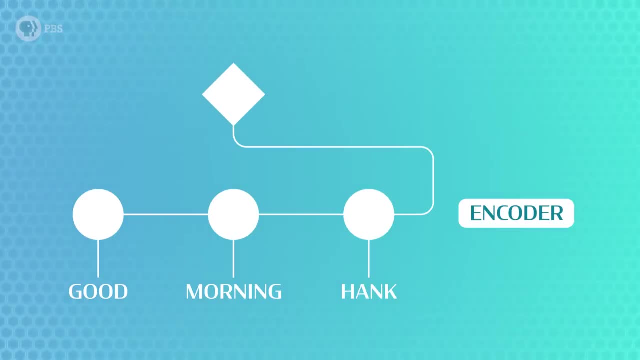 shared representation for the whole sentence. At this point our representation might be gibberish, but in order to train the RNN, we need it to make predictions For this particular problem. we'll consider a very simple decoder, a single-layer network. 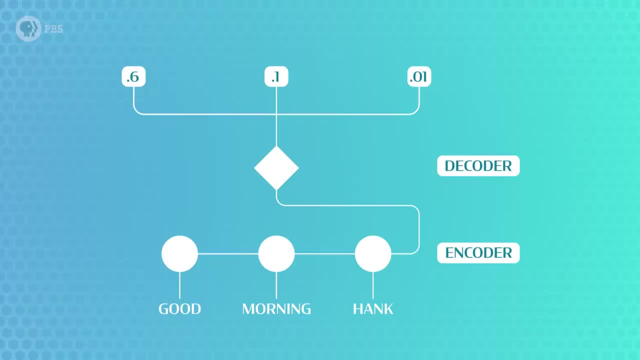 that takes in the sentence representation vector and then outputs a score for every possible word in our vocabulary. We can then interpret the highest-scored word as our model's prediction. Then we can use backpropagation to train the RNN, like we've done before with neural. 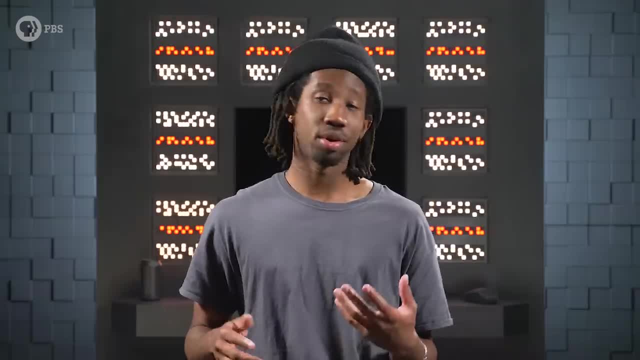 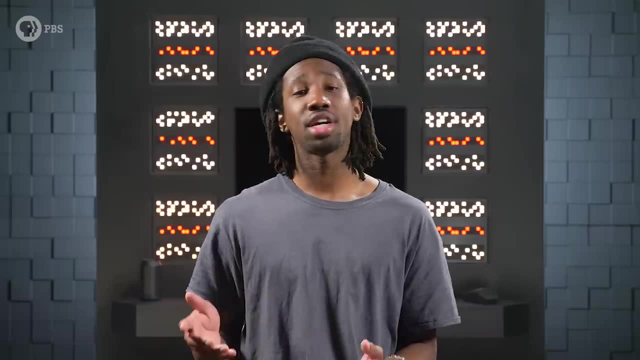 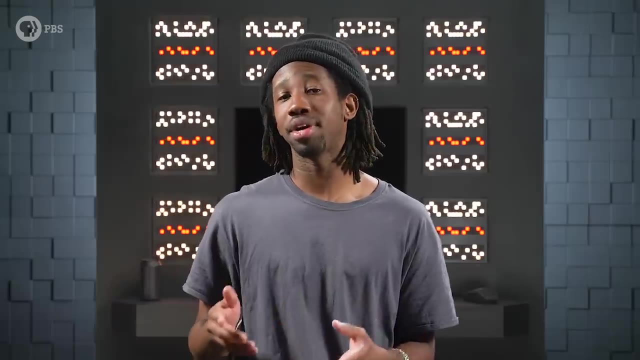 networks in Crash Course AI. So by training the model on which words to predict. next, the model learns weights for the encoder RNN and the decoder prediction layer. Plus the model changes those random representations we gave every word at the beginning. Specifically, if two words mean something similar, the model makes those vectors more. 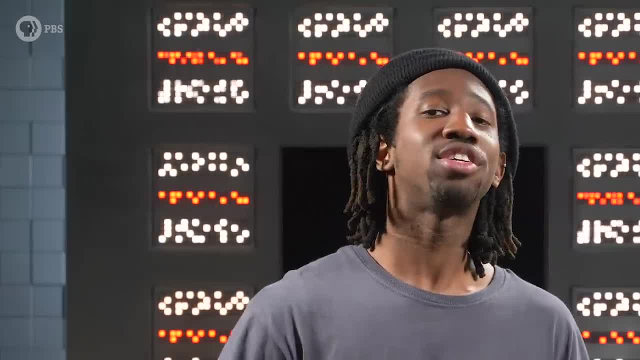 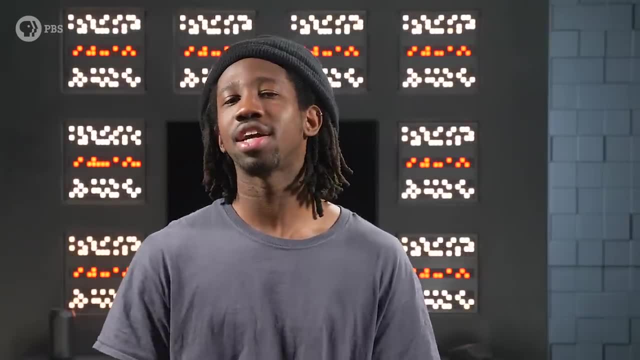 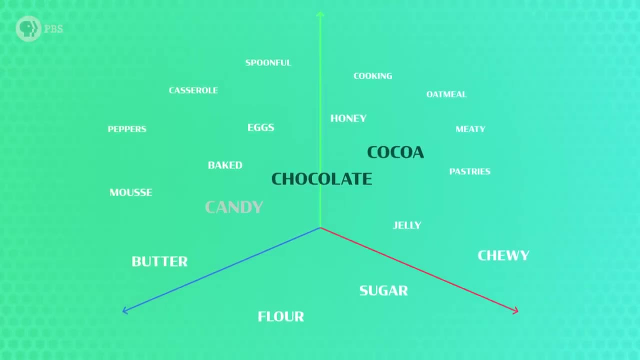 similar. By using these vectors to help make a plot, we can actually visualize word representations. For example, earlier we talked about chocolate and physics, So let's look at some word representations that researchers at Google trained Near chocolate. we have a lot of foods like coca and candy. 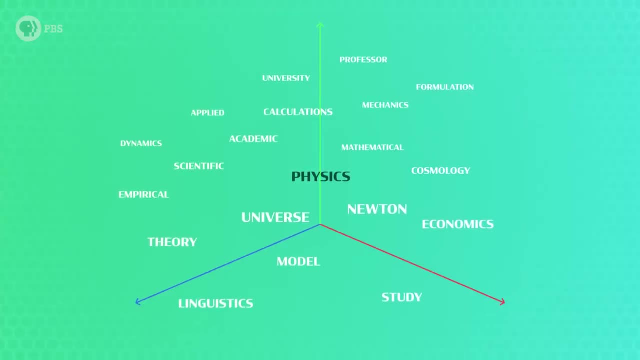 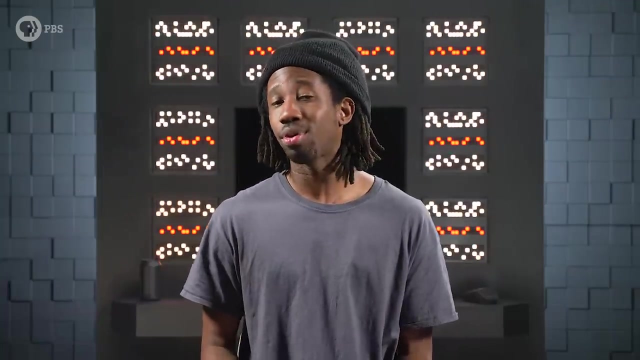 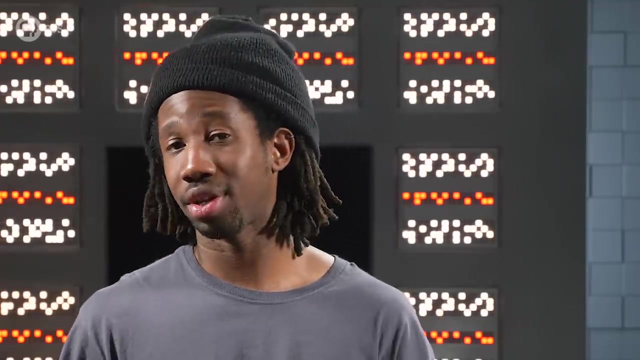 By comparison, words with similar representations to physics are Newton and universe. This whole process has used unsupervised learning and it's given us a basic way to learn some pretty interesting linguistic representations. But taking in part of a sentence and predicting the next word is just a tip of the iceberg. 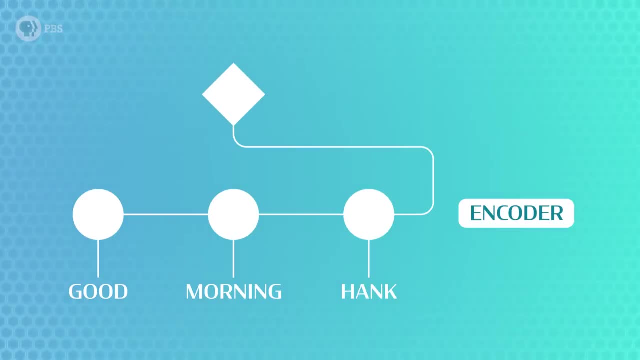 shared representation for the whole sentence. At this point our representation might be gibberish, but in order to train the RNN, we need it to make predictions For this particular problem. we'll consider a very simple decoder, a single-layer network. 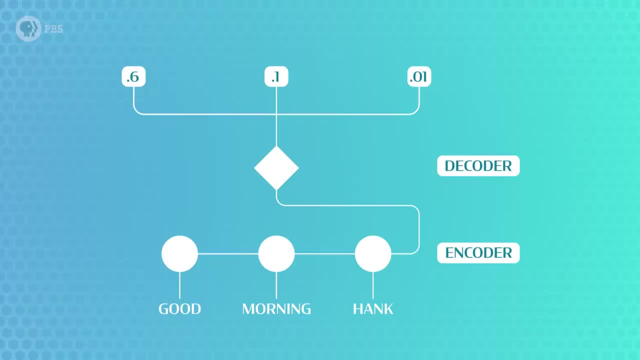 that takes in the sentence representation vector and then outputs a score for every possible word in our vocabulary. We can then interpret the highest-scored word as our model's prediction. Then we can use backpropagation to train the RNN, like we've done before with neural. 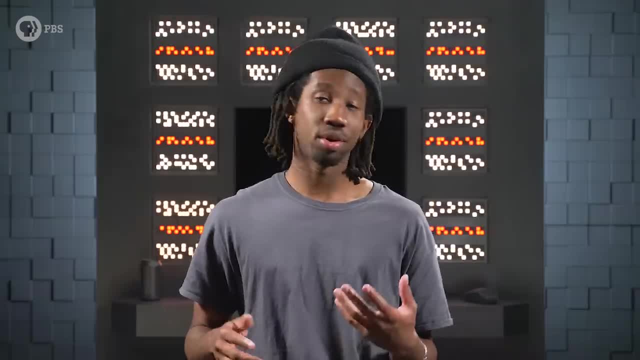 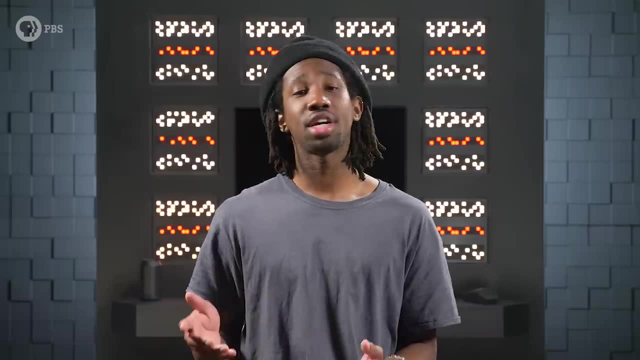 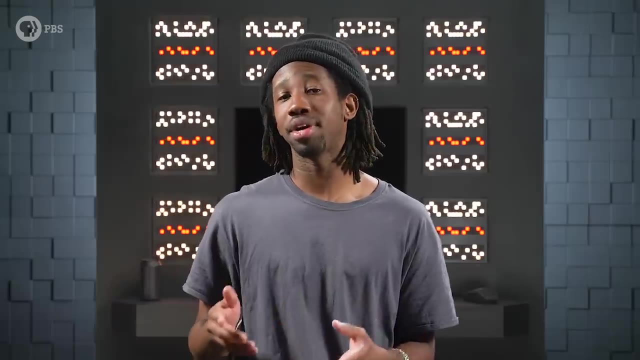 networks in Crash Course AI. So by training the model on which words to predict. next, the model learns weights for the encoder RNN and the decoder prediction layer. Plus the model changes those random representations we gave every word at the beginning. Specifically, if two words mean something similar, the model makes those vectors more. 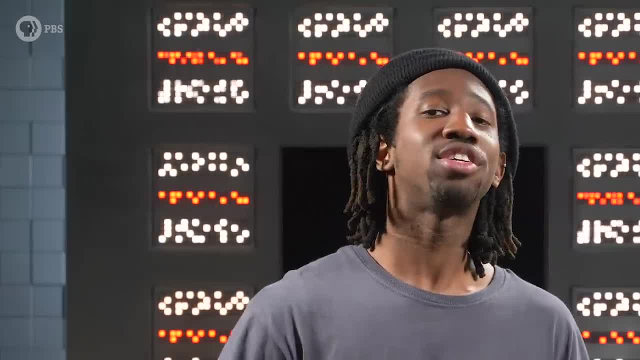 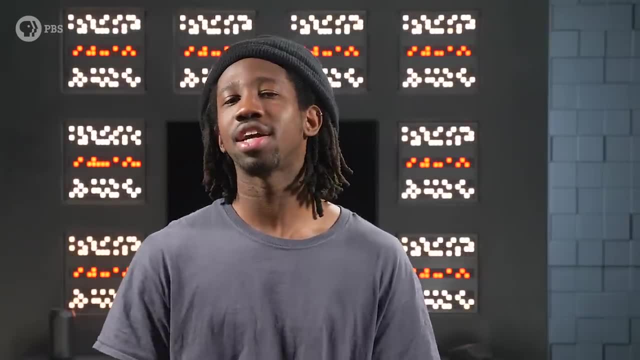 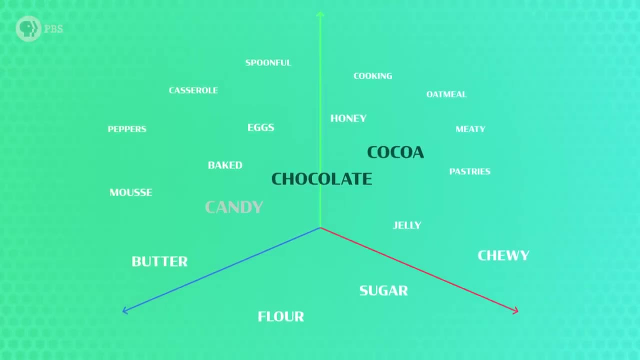 similar. By using these vectors to help make a plot, we can actually visualize word representations. For example, earlier we talked about chocolate and physics, So let's look at some word representations that researchers at Google trained Near chocolate. we have a lot of foods like coca and candy. 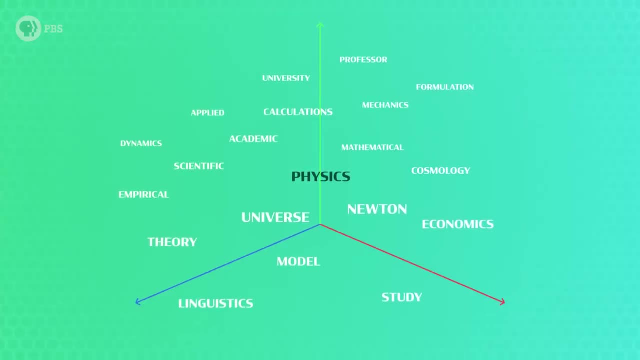 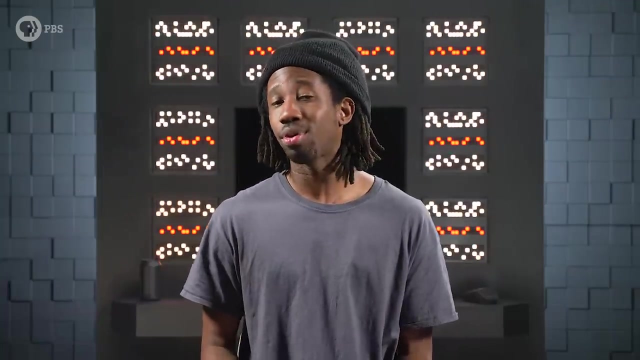 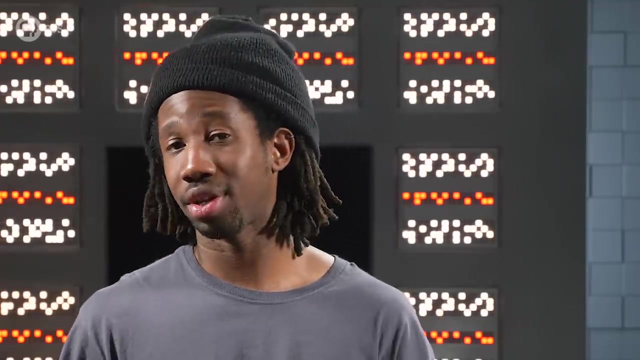 By comparison, words with similar representations to physics are Newton and universe. This whole process has used unsupervised learning and it's given us a basic way to learn some pretty interesting linguistic representations. But taking in part of a sentence and predicting the next word is just a tip of the iceberg. 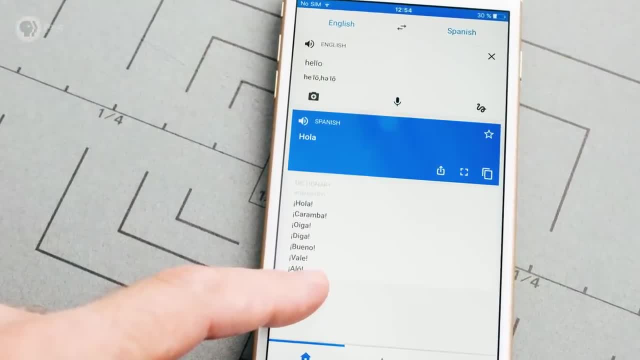 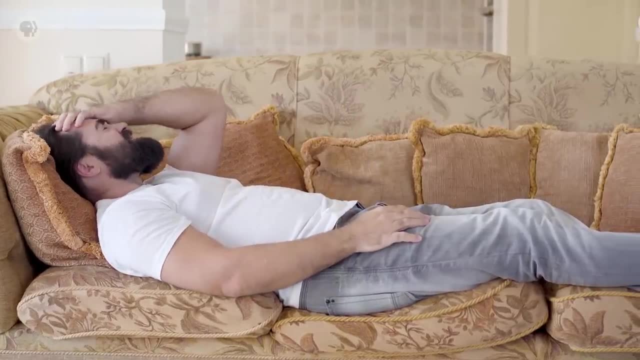 for NLP. If our model took in English and produced Spanish, we'd have a translation system. Or our model could read questions and produce answers, like Siri or Alexa try to do. Or our model could convert instructions into actions to control a household robot. 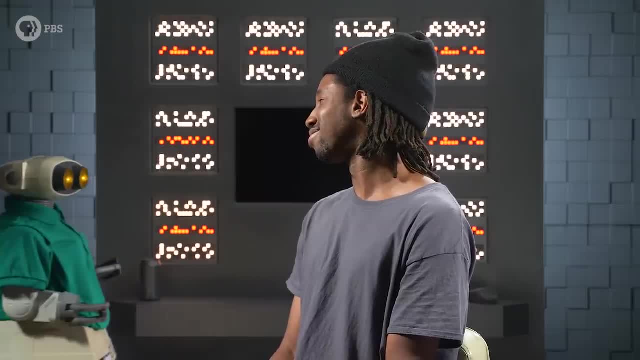 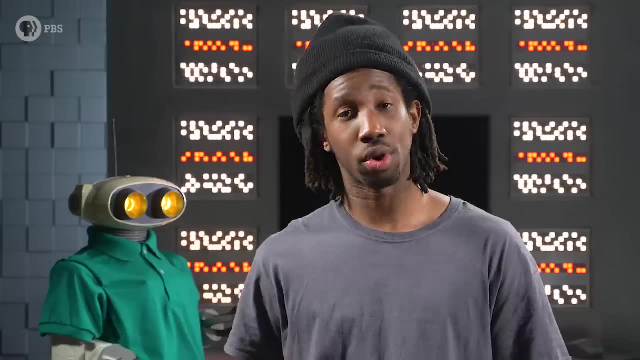 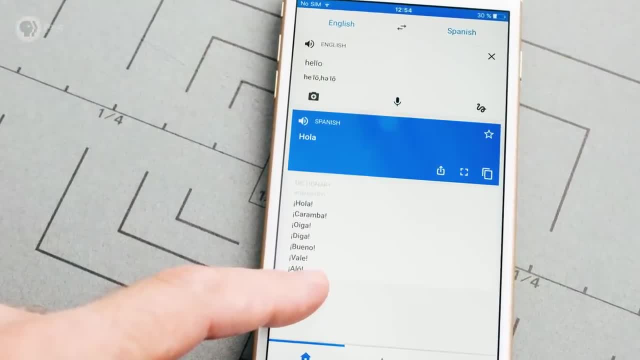 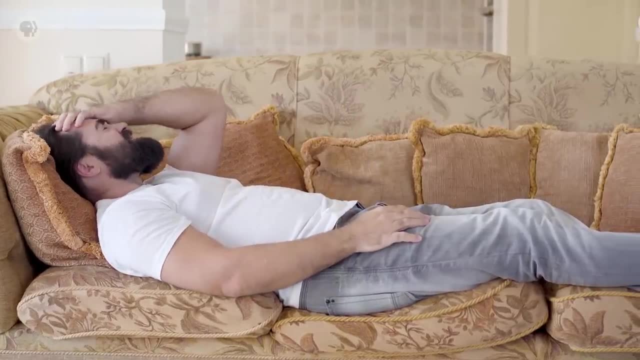 for NLP. If our model took in English and produced Spanish, we'd have a translation system. Or our model could read questions and produce answers, like Siri or Alexa try to do. Or our model could convert instructions into actions to control a household robot. 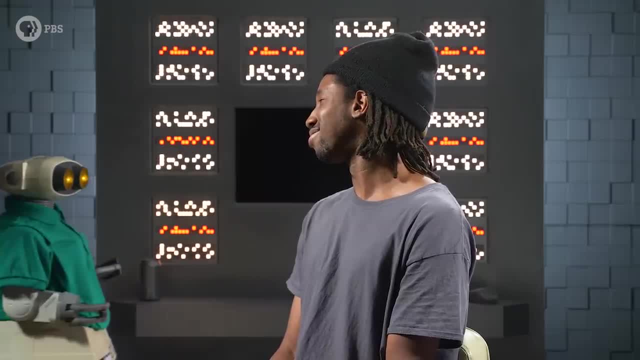 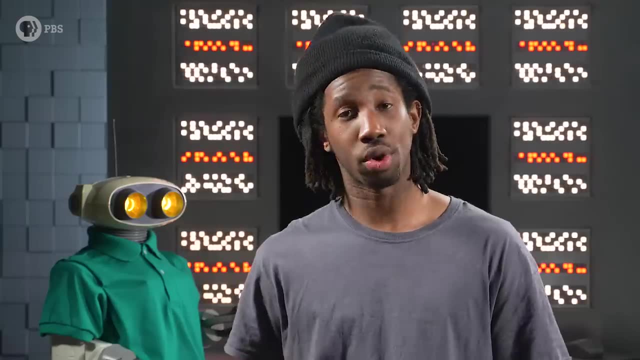 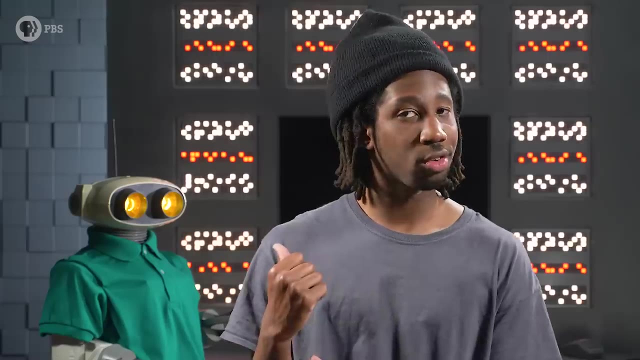 Hey, John Green Bot Just kidding. No, No, No, You're your own robot. Nobody controls you. But the representation of words that a model learns for one kind of task might not work for others, Like, for example, if we train John Green Bot by having him read a bunch of cooking. 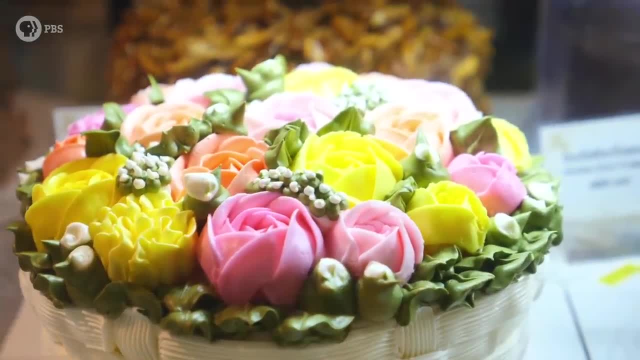 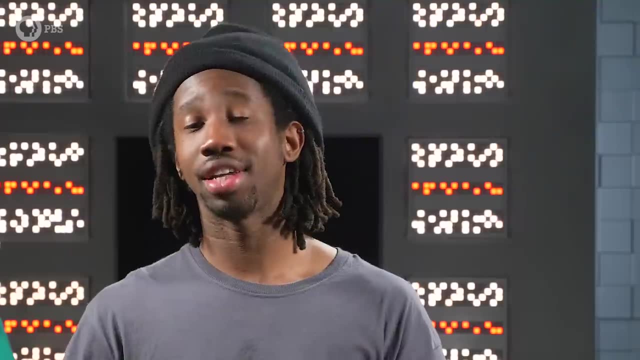 recipes. he might learn that roses are made of icing and placed on cakes, But he won't learn that cake roses are different from real roses that have thorns and make a pretty bouquet. Acquiring, encoding and using written or spoken knowledge to help people is a huge 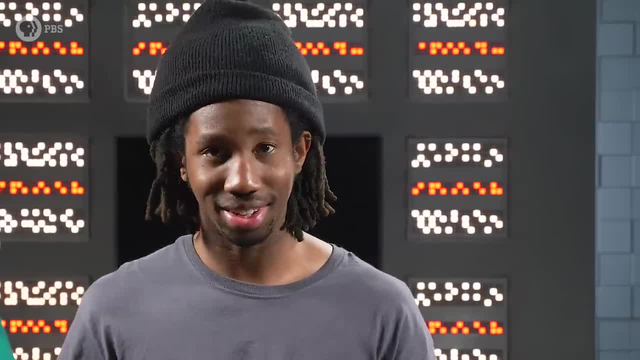 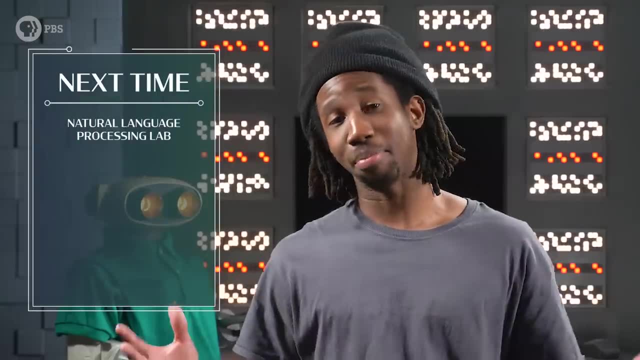 and exciting task, Because we use language for many things. Every time you type or talk to a computer, phone or other gadget, NLP is there. Now that we understand the basics, next week we'll dive in and build a language model. 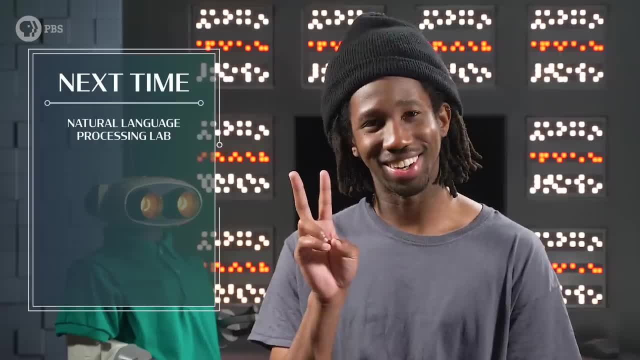 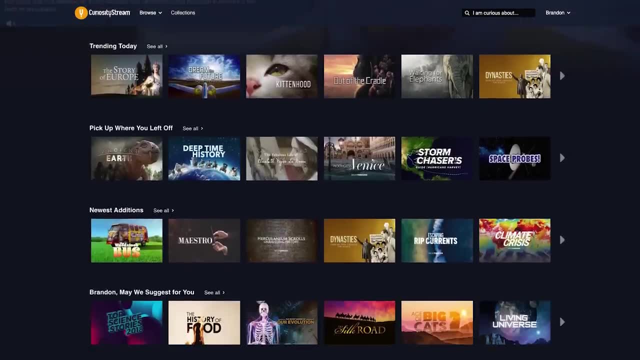 together for John Green Bot in our second lab. See you then. Thank you to CuriosityStream for supporting PBS Digital Studios. CuriosityStream is a subscription streaming service that offers documentaries and nonfiction titles from a variety of filmmakers, including CuriosityStream Radio. 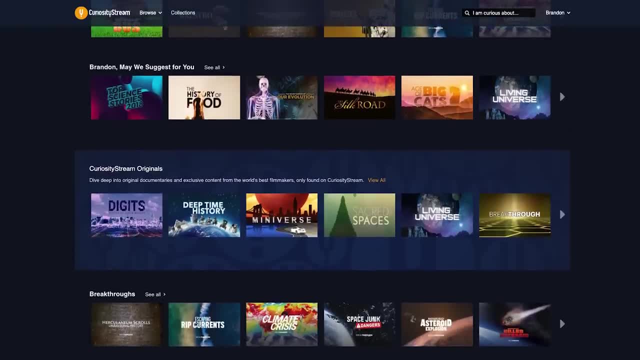 If you want to learn more about CuriosityStream, check out CuriosityStreamcom. CuriosityStream is a subscription streaming service that offers documentaries and nonfiction titles from a variety of filmmakers, including CuriosityStream Radio. Link will be in the description. 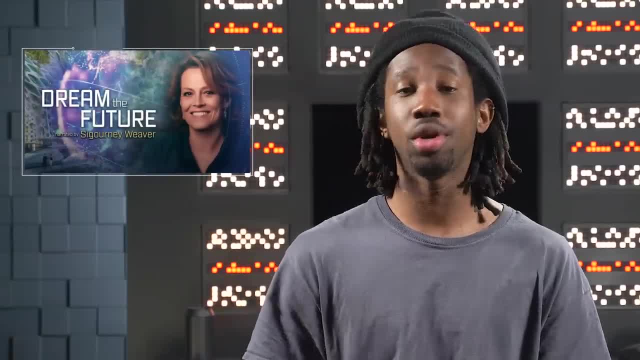 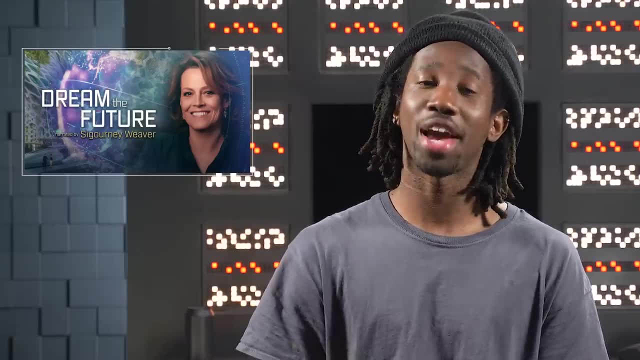 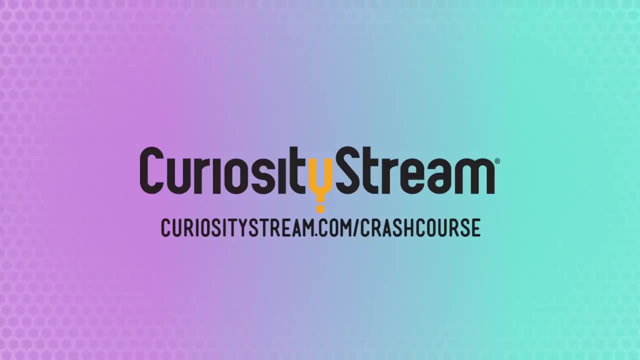 For example, you can stream Dream the Future, in which host Sigourney Weaver asks the question what will the future look like? as she examines how new discoveries and research will impact our everyday lives in the year 2050.. You can learn more at CuriosityStreamcom. slash crash course or click the link in the. 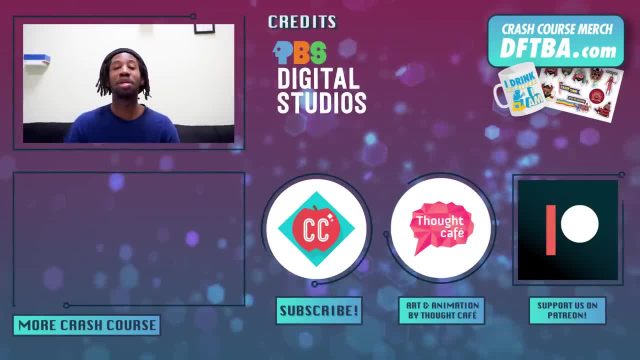 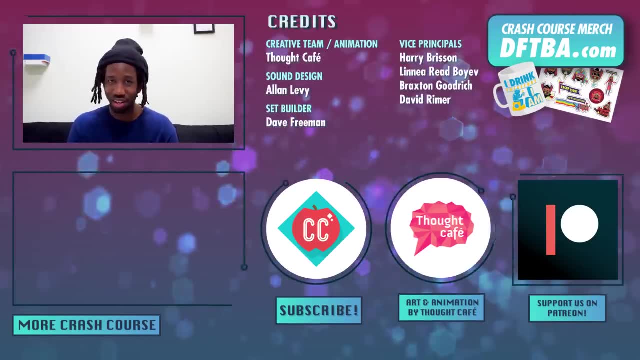 description: Crash Course AI is produced in association with PBS Digital Studios. If you want to keep Crash Course free for everyone forever, you can join our community on Patreon, And if you want to learn more about how human brains process language, you can check out. this video from Crash Course Psychology. 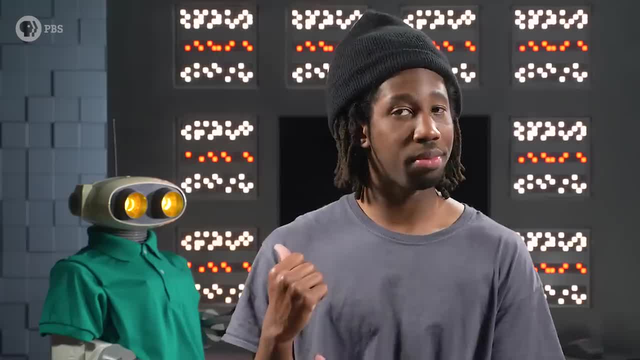 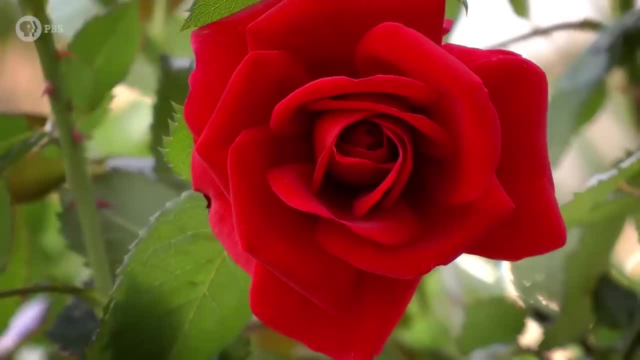 for others, Like, for example, if we trained John Green Bot by having him read a bunch of cooking recipes, he might learn that roses are made of icing and placed on cakes, But he won't learn that cake roses are different from real roses that have thorns and make.